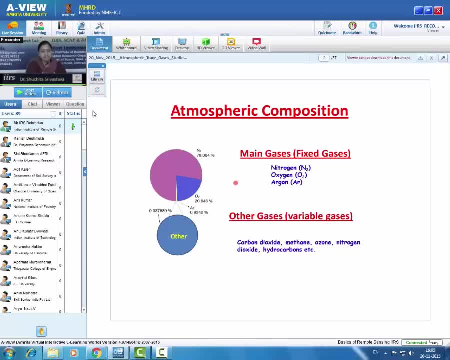 will not change. Remaining 0.03% contains all the other gases in the atmosphere. This is very small amount and it contains more than 1000 gases. These gases are called variable gases- Variable gases because their concentration vary significantly with space and time, Though these gases are 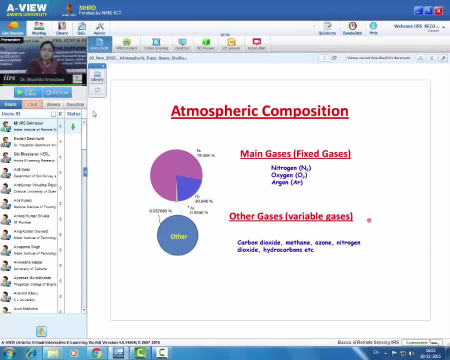 very small in amount. these few of these gases play very important role in the life of the earth, very important role in the atmosphere. Few examples are carbon dioxide, methane, ozone, nitrogen dioxide and hydrocarbons. Few of these gases can act as greenhouse gases. 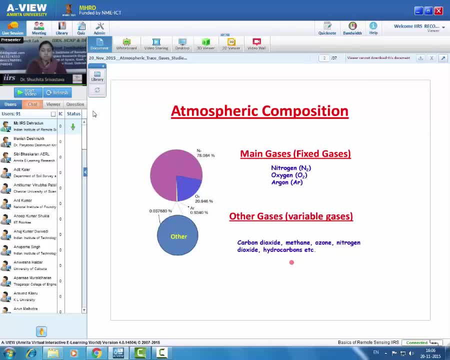 Greenhouse gases are those gases which absorb terrestrial infrared radiation and contribute for the radiative budget of earth. Few gases can act as pollutants. Few gases can act as oxidants. So these are variable gases which vary with space and time, but having very important. 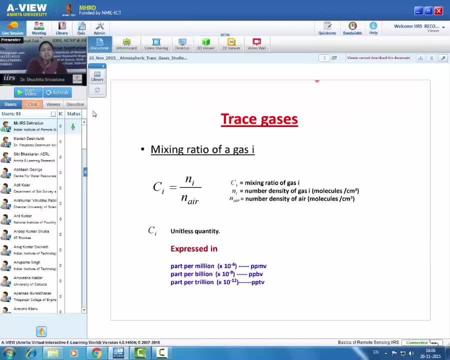 implication in earth's climate. As these gases are very small in amount, we cannot express these gases in percentage Like if ozone is very ozone concentration is in percentage- it is 0.0000003 percent- then it is not a convenient way to express these gases. So these are variable gases which vary with space and time. but having 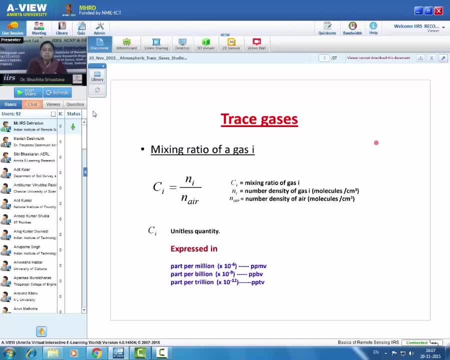 very important implication in earth's climate. So these are variable gases which vary with space and time, but having very important implication in earth's climate. So these are variable gases which vary with space and time, but having very important implication in earth's climate. For that we, we we use mixing ratio of a gas, Here c i is equal to ni by n air, where ni is the number. 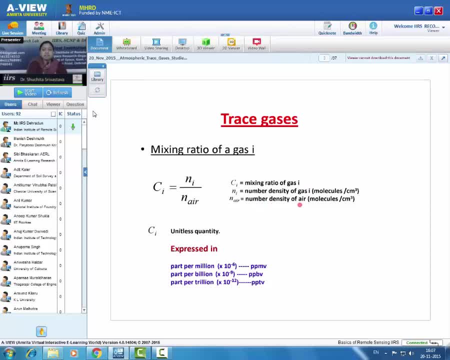 density of a particular gas i to the number density of air, Then c i will be mixing ratio of that particular gas i. As you can see, it is a unitless quantity. This quantity is expressed in terms of part per million, part per billion or part per trillion. It depends on the amount of gas present. 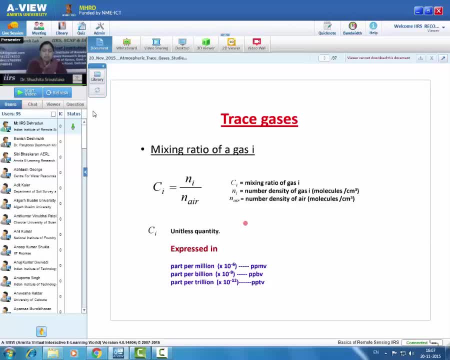 Suppose we are talking about ozone and this ratio for ozone comes is equal to 0.3 into 10 to the power minus 9.. In that case it will be said that this gas is present in the amount of 0.3 ppbv. 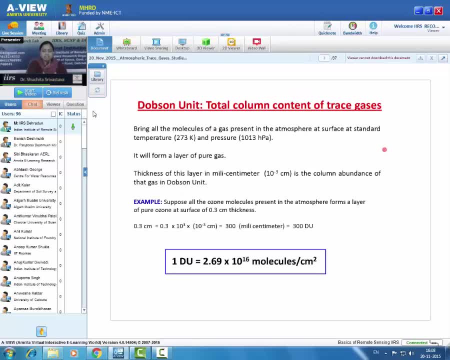 Other important unit of measuring trace gases is Dobson unit. This is a unit which is in which total column content of gases are expressed. For expressing any gas in Dobson unit you have to bring all the molecules of this gas present in the atmosphere at surface at standard temperature. 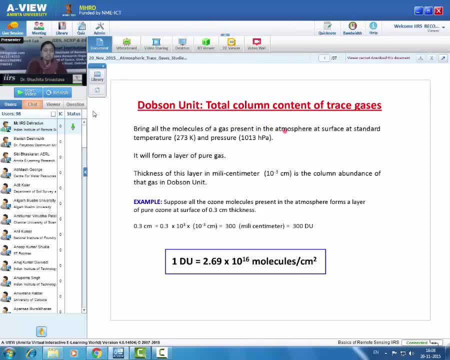 and pressure. Standard temperature: 273 degree Kelvin. and standard temperature: 273 degree Kelvin. pressure: 1013 hectopascal. Then it will form a layer of pure gas. Thickness of this layer in millisentimeter is the column abundance of that gas in Dobson unit. To understand this, a simple 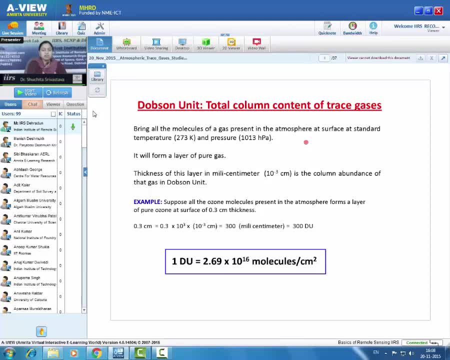 example is given. Suppose all the ozone molecules present in the atmosphere from surface to top of the atmosphere. We have bring all the gas molecules near the surface and it forms a layer of pure ozone of the thickness 0.3 centimeter, which can be written as 0.3 centimeter can be. 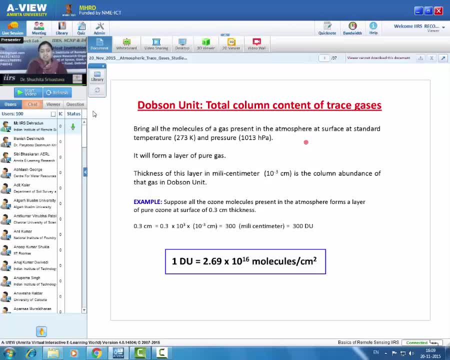 written as 300 millisentimeter, Then it will be 300 Dobson unit, because it is thickness, is expressed in millisentimeter. One Dobson unit contains 2.69 into 10 to the power, 16 molecules per centimeter square. 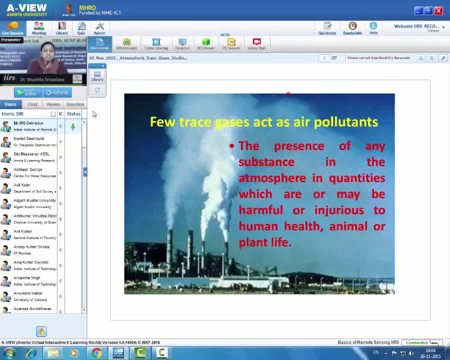 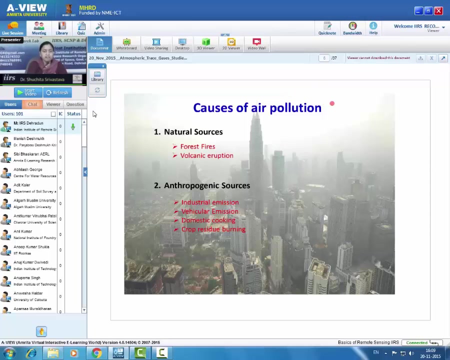 few trace gases can act as air pollutants. the question is: what is air pollution? the presence of any substance in the atmosphere in quantities which are, or may be, harmful or injurious to human health, animal or plant life. there are two type of sources in the atmosphere for this sort of air pollution. one is natural source and two anthropogenic source. natural- 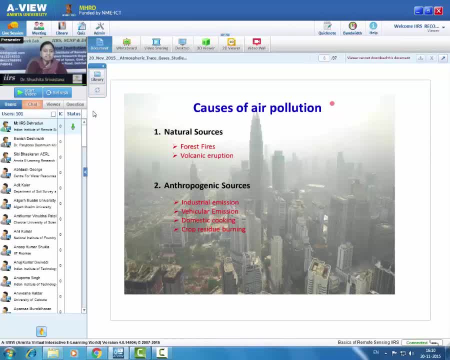 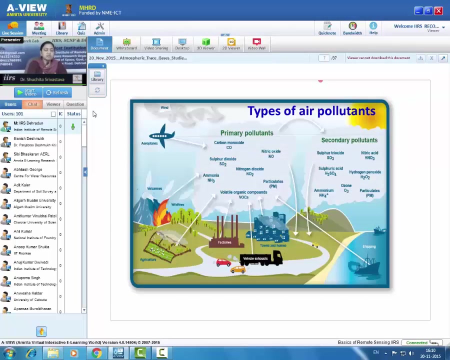 sources are those sources which are naturally occurred in the era in our earth, like forest fire or volcanic eruption. anthropogenic sources are those sources which are man-made, like industrial emission, vehicular emission, domestic cooking, crop residue, burning, etc. there are two type of air pollutants present in the atmosphere. one is primary pollutant, which are directly 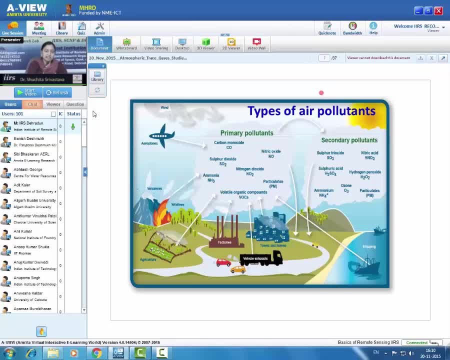 emitted and stare demasiado lada are two types of air pollutants present in the atmosphere. one is primary pollutant, which are directly emitted and stored within the atmosphere' in the atmosphere because of any natural or anthropogenic activities. The few examples are given here. These are carbon monoxide, nitric oxide, sulfur dioxide, nitrogen dioxide, volatile. 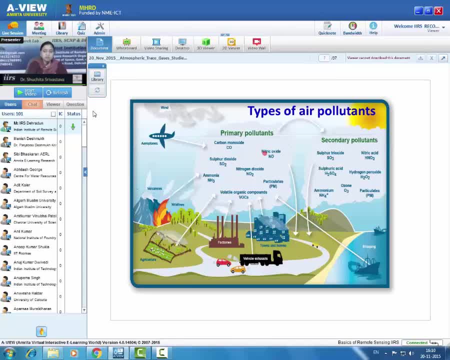 organic compounds, particulate matter, ammonia, etc. These primary pollutants can, because of complex chemistry or photochemistry, generate secondary pollutants. Secondary pollutants are not directly emitted. They are produced by primary pollutants and having very bad impact on human health or crop production. These are sulfuric acid, nitric acid, ozone, hydrogen peroxide, etc. 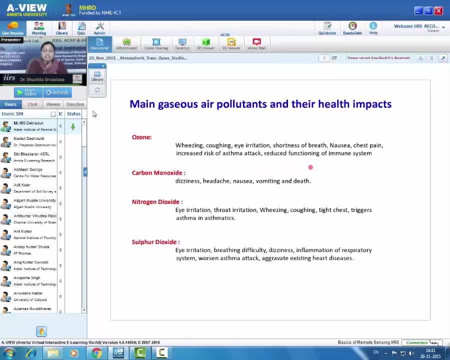 Main gaseous air pollutants are given here and their health impacts are also written. Like ozone can cause wheezing, cough and cough. These are the main pollutants. These are the main pollutants: Eye irritation, shortness of breath, nausea, chest pain, increased risk of asthma attack. 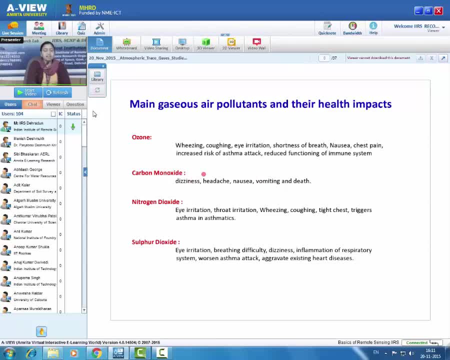 reduced functioning of immune system, etc. Carbon monoxide can create dizziness, headache, nausea, vomiting and death. Nitrogen dioxide can create eye irritation, throat infection, wheezing, coughing. tight chest triggers asthma and asthmatics. 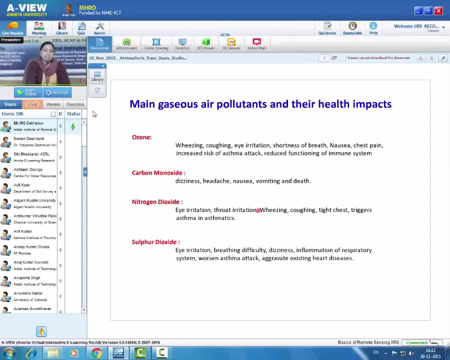 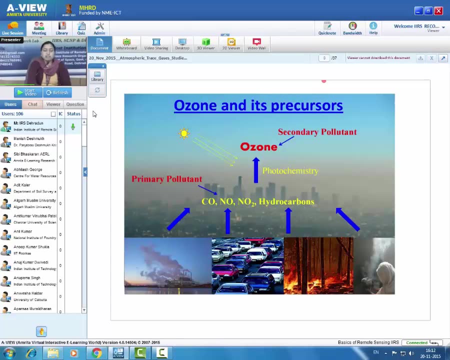 Sulphur dioxide can create eye irritation, breathing difficulty, dizziness, inflammation of respiratory systems versus asthma attack, aggravate existing health heart diseases. So in the present lecture we will focus mainly on ozone and its precursors. Precursors of ozone. 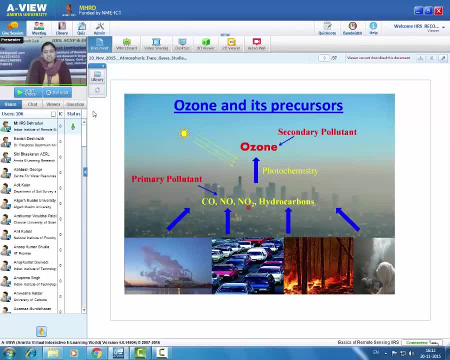 are carbon monoxide, nitric oxide, nitrogen dioxide and hydrocarbons. These, all these gases are pollutants and emitted in the atmosphere because of industrial emission, vehicular emission, biomass burning or domestic cooking. As I already told that, these are those gases which are directly 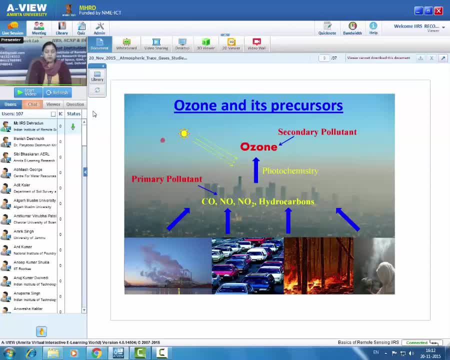 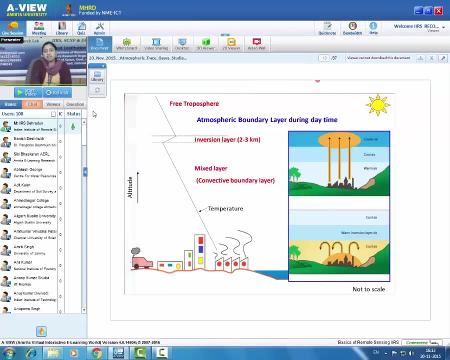 emitted in the atmosphere. these are primary pollutants. These pollutants, because of very complex chemistry, in the presence of sunlight creates ozone, So ozone is a secondary pollutant, Once emitted. there are several atmospheric parameters which can affect the distribution of these gases over one location. The most fundamental atmospheric process which affects 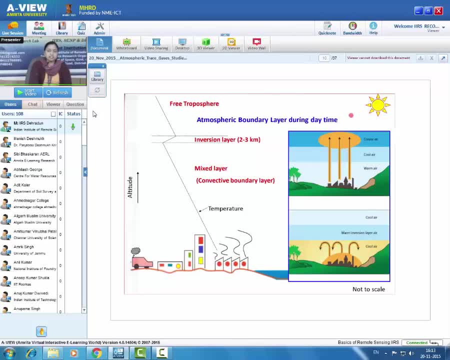 distribution of air pollutant over one location is atmospheric boundary layer. What is atmospheric boundary layer? Atmospheric boundary layer is the lowest part of the troposphere which directly responds to surface forcing. Like, if air pollution is emitted near the surface, within an hour it will be mixed within the boundary. 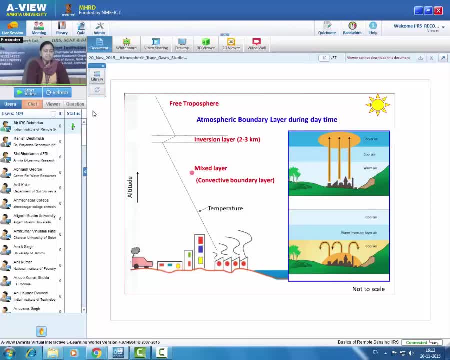 layer. However, it can take several days to get mixed up within the other free troposphere. So what defines the boundary layer? The top of boundary layer is there is always a inversion layer. because of in this inversion layer, temperature slightly increases and this differentiates between boundary layer and the free troposphere. 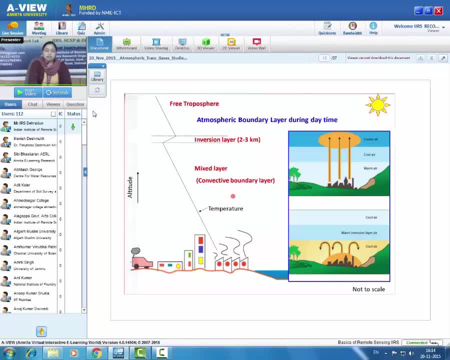 oppressor And this boundary layer is very important for the distribution of air pollutants. Suppose a pollution plume is emitted inside this particular boundary layer and because Earth becomes warmer during daytime, this performed volume, this partial, will move towards the upper side because it is warmer with respect to ambient air And in that case it will be lighter than. ambient air and it will move towards the, towards higher altitude, As suppose if something gets higher then it gets softer, more rigid. Nevermniej, higher, higher air will, because very will get a higher and heavier layer And in that case it will be warmer with respect to ambient air and it willutz higher, which would increase the pollen layer and will reduce the dryness of it. 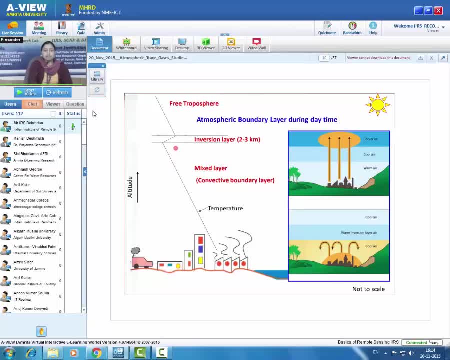 the towards higher altitude, it will move till it finds a layer which is warmer. with respect to this, it is similar to a balloon which is filled of hot air. as long as balloon contains hotter air, it will go higher. similarly, as long as parcel containing pollution is warmer with respect to ambient air, it will move. 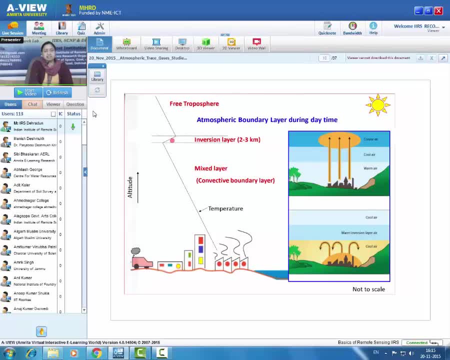 higher, but near, in this inversion layer. the air parcel present inside this inversion layer is always warmer with respect to air which is just present just below this inversion layer. so this layer will act as a barrier. it will not allow this air parcel to cross it and go inside the pre troposphere. so height of 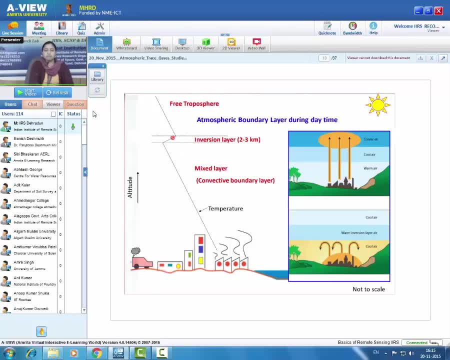 atmospheric boundary layer defines a barrier for the mixing of air polytechs. height of atmospheric boundary layer varies with space and time. during daytime, boundary layer varies with space and time. during daytime, boundary layer varies with space and time. layer height is maximum around 12 o'clock to 2 o'clock and its height is very small during. 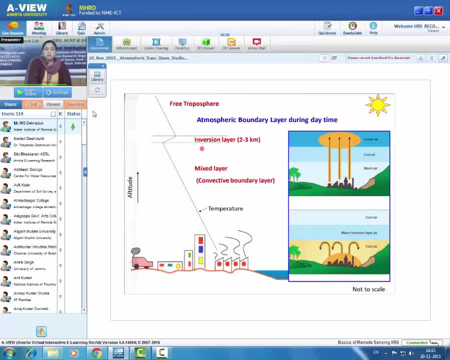 night time. Similarly, the boundary layer height is high during summer time and it is low during winter time. Suppose there is no inversion layer, then what will happen? The example is given in this picture. This is air pollution which is emitted over one location and there is warm air. 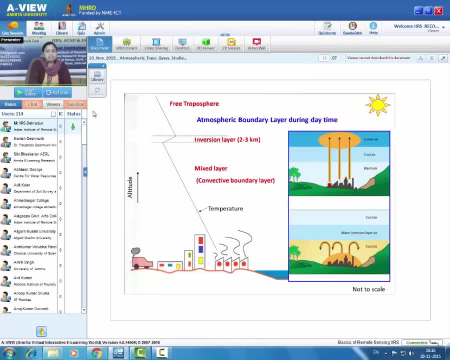 then cool air and then cooler air. So there is no inversion layer. Air pollution will keep on moving towards the higher altitude and it can go up to tropopause. But if there is a inversion layer present, then this inversion layer will act as a barrier and it will not allow this pollution. 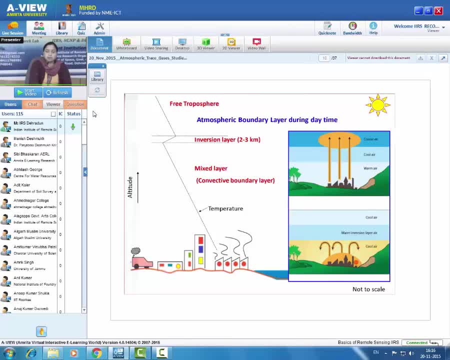 to penetrate through this. In that case, the pollution will be trapped. The lower the height of inversion layer, the lower the height of air pollution, the higher the air pollution will be. If there is no inversion layer, whatever pollution is emitted that will keep on moving towards the. 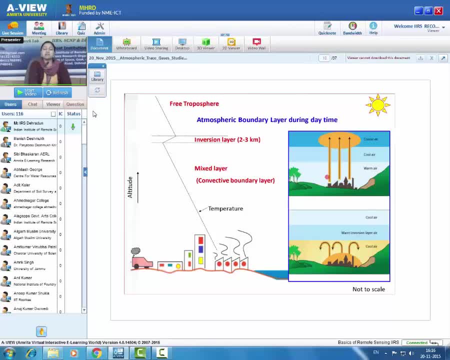 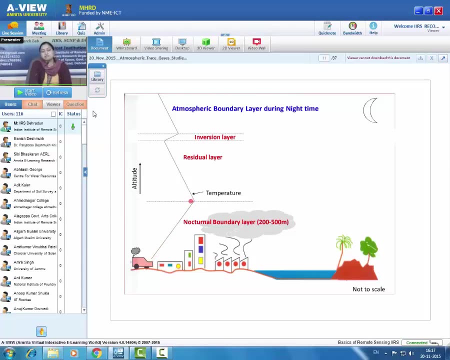 high altitude and the air quality over the region will become very, very good. So boundary layer plays a very important role for the air quality over one region. During night time, earth surface becomes cooler and temperature structure near the surface becomes different. It now near the surface, from surface to around 200 to 500 meter, temperature increases Again. this is 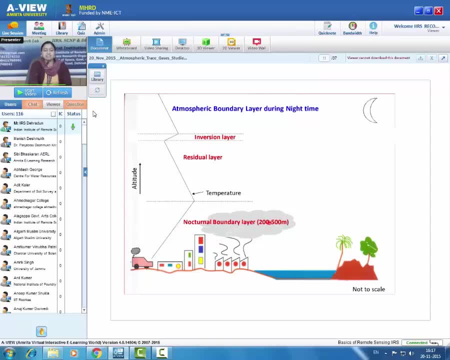 a inversion layer. Because of this inversion layer, whatever pollution emitted near the surface will remain trapped. There will not be any vertical movement. There can be only horizontal movement or forced wind movement, But this because this parcel is all the parcel, which is which is sitting. 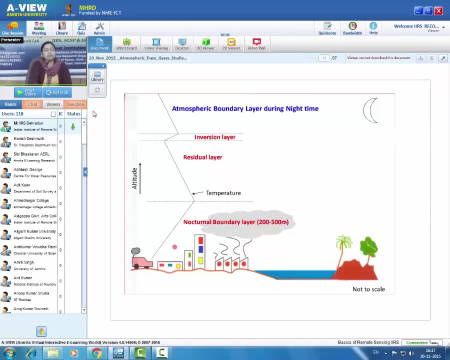 on high altitude. So this is a inversion layer. So this is a inversion layer. So this is a inversion layer. The higher side is warmer, so there will not be vertical movement. So during night time, if the pollution is emitted in the atmosphere, that will remain trapped. So if pollution is emitted in the 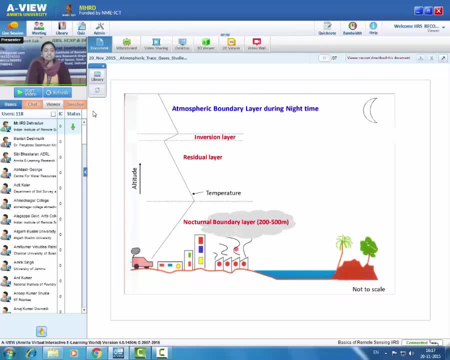 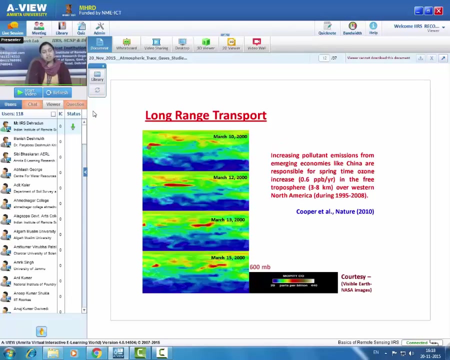 atmosphere. during night time, air quality over that region can be significantly poor. Above the nocturnal boundary layer, daytime residual air occurs, which is just the remaining part of the vertically mixed layer, and inversion layer also remains like that. Other than that, other than local effect, there can be long range transport of air pollutants. 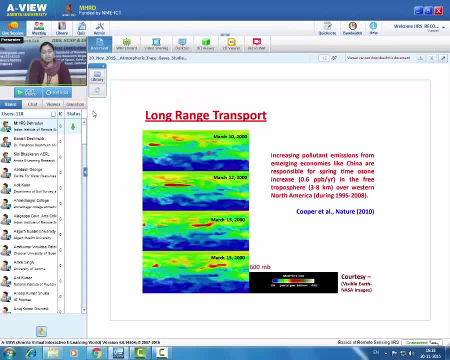 Once emitted, these pollutants can get transported to large distances, like an example is shown here, where data is taken from Moppet instrument for carbon monoxide at 600 millibar, And this data, this carbon monoxide, varies from 20 to 440 part per billion. This plot is for 5 consecutive. 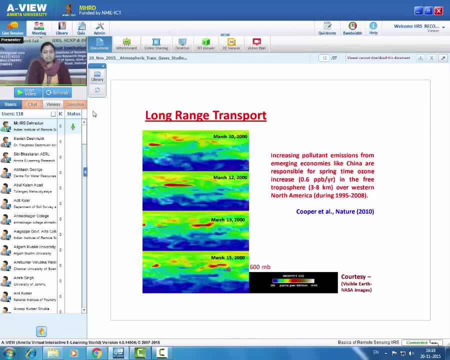 is March 10,, March 12,, 13 and 15, and this shows that over this location, China, a pollution plume of carbon monoxide emitted and within five days it got transported to northern America. So it is not necessary that a place will be polluted if, and only if, over that location. 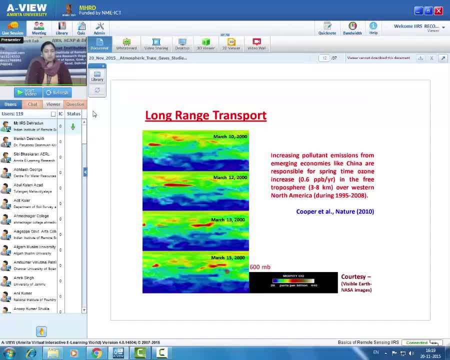 the pollution is emitted. It is also possible that the region where this pollution is not emitted it can receive pollution from upwind locations, So monitoring of upwind location air quality is also very important. A very good study shows that increasing pollutant emissions from emerging economies like China are responsible for springtime ozone increase. 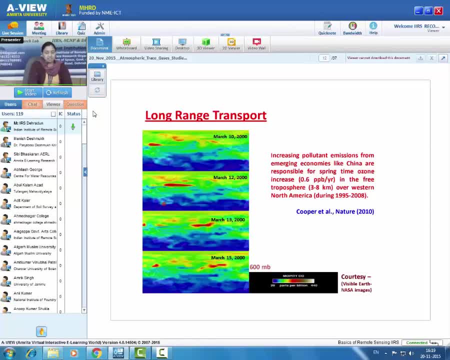 in the form of carbon monoxide emission. So the昨 night's water pollution detection of the air quality is also very good. A very good study shows that increasing pollutant free troposphere over western north america, so continuous emission over upwind location, can. 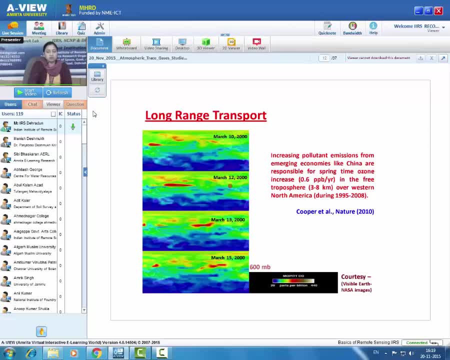 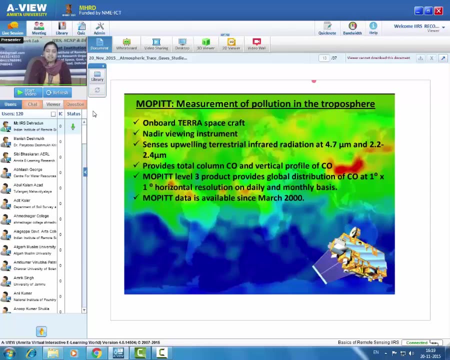 significantly degrade air quality over the downwind location. this law, this: when we want to study long-range transport, you should have consecutive data at the same time, data all over the globe. that data can be provided by satellite. only few satellite instruments are introduced here. one of them is moped measurement of pollution in the troposphere. it is an instrument on board. 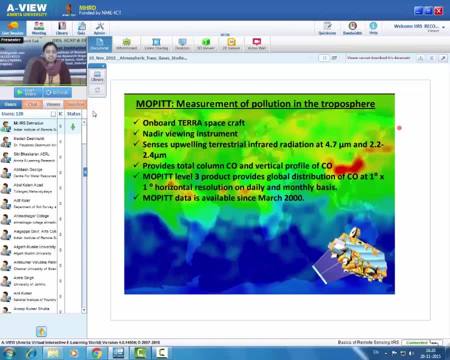 terra spacecraft. it is a nadir viewing instrument. it senses a paling terrestrial infrared radiation at 4.7 micrometer and 2.2 to 2.4 micrometer. it provides total column content of carbon monoxide and its vertical profile it moped level 3 product. 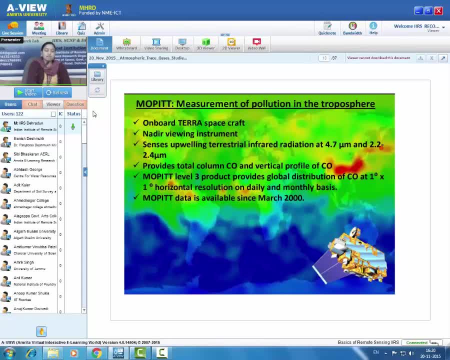 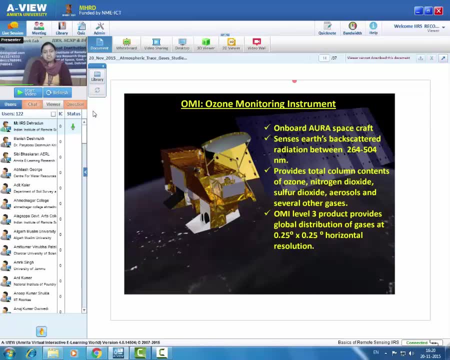 provides global distribution of carbon monoxide at one degree by one degree horizontal resolution, and this data is available since march 2000. another instrument: ozone monitoring instrument. this is an instrument on board aurai spacecraft. it senses earth's back scattered radiation between 264 to 504 nanometer. it provides total column content of several gases like ozone nitrogen. 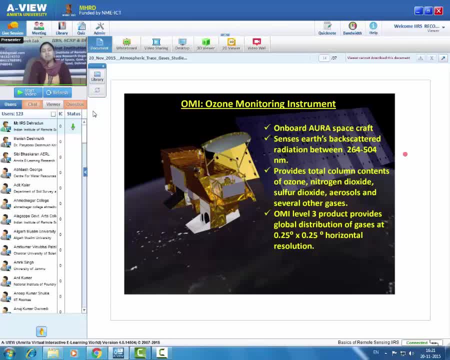 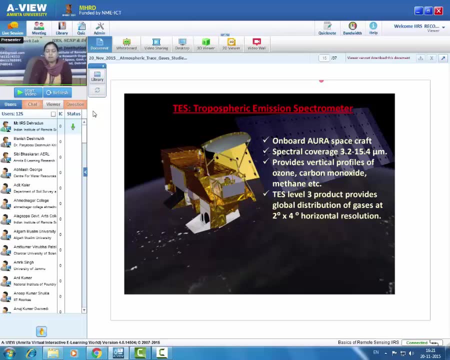 dioxide, sulfur dioxide, etc. omi level 3 product provides global distribution of gases at 0.25 for 0.25 degree horizontal resolution. another instrument: tropospheric emission spectrometer, commonly known as test. it is on board aurai spacecraft. its spectral coverage is 3.2 to 15.4 micrometer. it provides vertical profile of 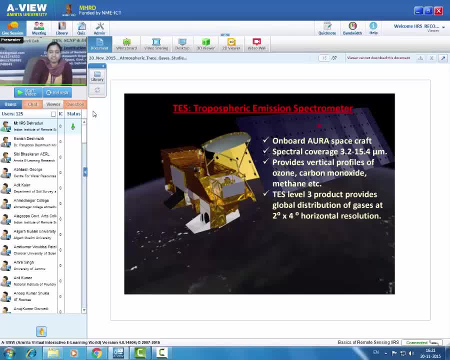 ozone, carbon monoxide, methane, etc. it is also known as a test. it is on board aurai spacecraft. its spectral coverage is 3.2 to 15.4 micrometer. it provides vertical profile of ozone, carbon monoxide, methane, etc. test level 3 product provides global distribution of gases at 2 cross 4 degree horizontal resolution. 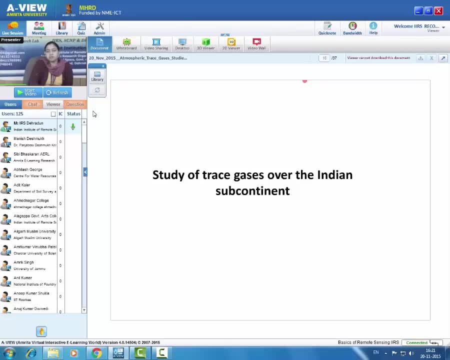 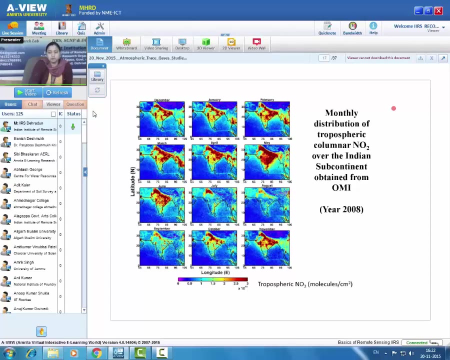 so to now, we will study this gas distribution over indian subcontinent and what are the atmospheric processes which are affecting the distribution of these gases. so here in this plot, monthly distribution of tropospheric columnar no2 is shown over the indian subcontinent, which is obtained from 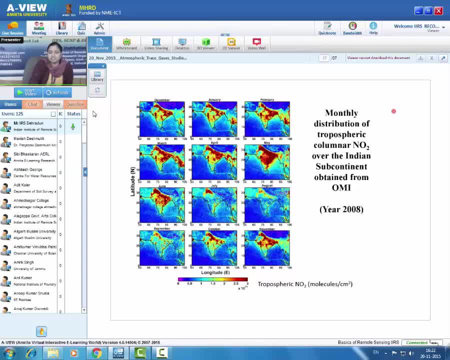 ozone monitoring instrument for year 2008. this plot is shown from december to december, january, february to september, october and november. this plot shows that total columnar content- tropospheric columnar content- of nitrogen dioxide- is high during december, january, february. 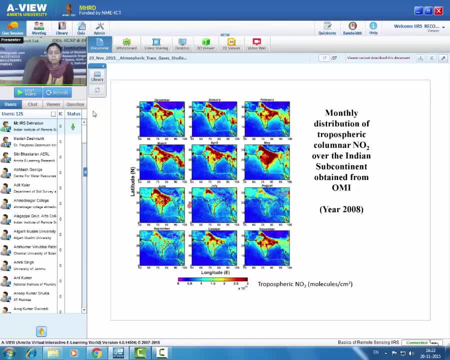 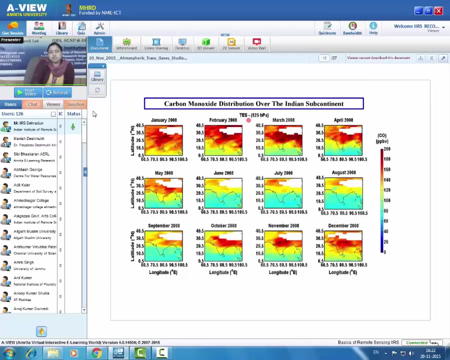 march, april, may and june, and after that this value is shown over the indian subcontinent- becomes lower and it remains lower till september. after that again october and november values are higher. similarly, we have also investigated distribution of carbon monoxide by obtained from tropospheric emission spectrometer at 825 hectopascal. this also shows similar type of 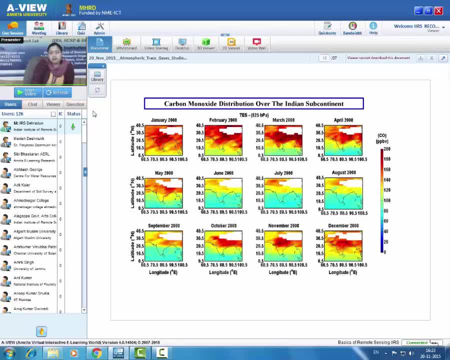 feature in which january, february, march, april and may and june and after that this value is shown over the indian subcontinent. values of carbon monoxide are high. june, july, august and september shows lower value, and again october, november and december shows higher value. and what is the reason why we are getting high? 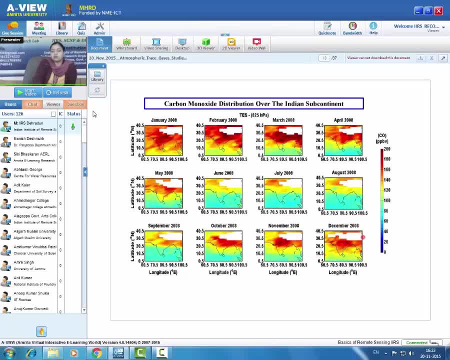 value during january to may and again in from october to december, and why we are getting lower value during june to september. so there are two type of possibilities, which we have already read: atmospheric boundary layer dynamics and the second is transport atmospheric boundary effect of. 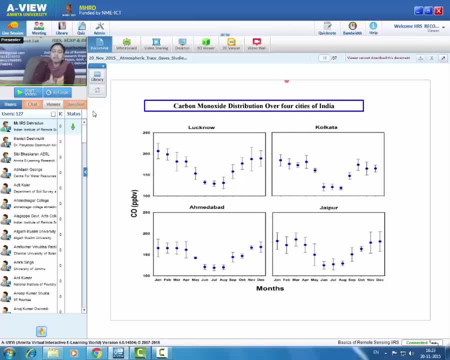 atmospheric boundary layer and transport can be studied when we take specific cities. so we have taken four cities over india. those are lucknow, kolkata, ahmedabad and jaipur. again, like the special plot, this plot also shows high value during winter and low value during summer. to 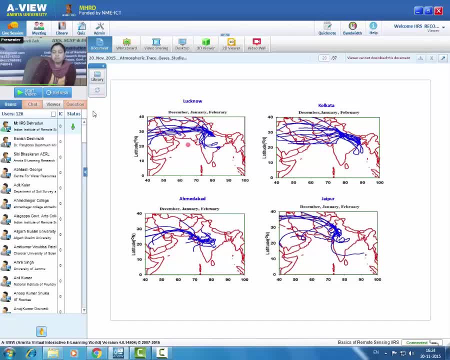 express to explain why we are getting this type of variation, we have calculated back trajectories. back trajectories are nothing but the latitude and longitude information back in time of a air parcel which is present on a one particular day over the observational location. so for this we have used 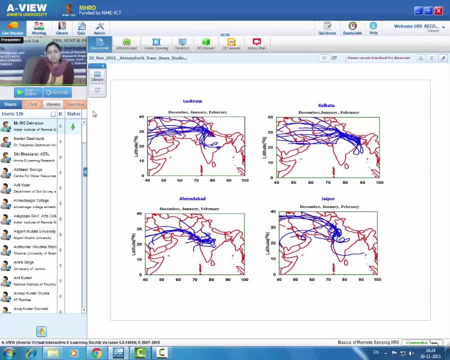 high speed back trajectory model, by using which we can calculate location of air parcel back in time. we, if we know what is the uh, if we know, we want to know what is the location of air parcel today, then we can track it back. suppose one air parcel is present over dehradun today, then what was its? 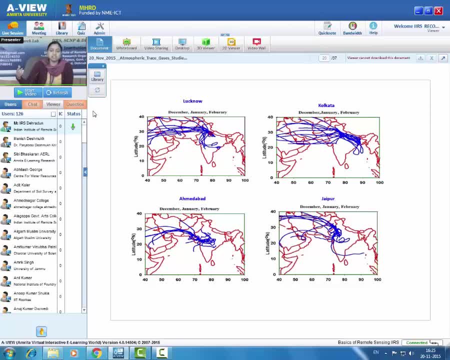 location before one day, what was its location before today, and so on, can be calculated using trajectory models. so in this plot we have taken seven days back trajectory over lucknow, kolkata, ahmedabad and jaipur during december, january and february. plot shows that in this, all these locations are receiving air parcel from the continental 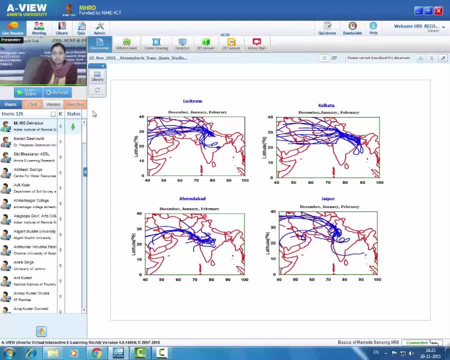 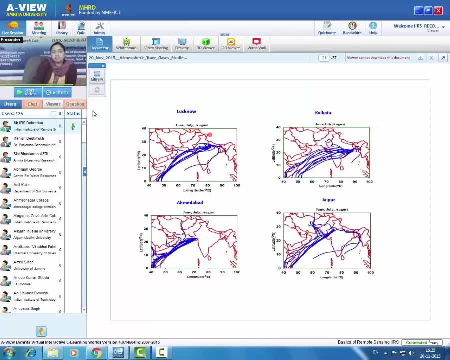 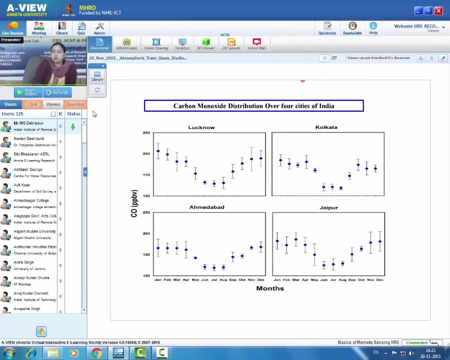 region, either from Middle East or Pakistan, and or it is circulating over the Indian region itself. however, during June, July and August, these air parcels are arriving from oceanic region, from Indian Ocean via Arabian Sea. so this shows that during winter time we are receiving air mass from anthropogenic polluted locations, whereas during summer time we are receiving 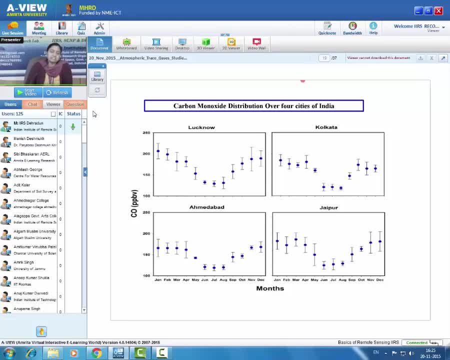 air parcel from the cleaner marine region. when air is coming from cleaner marine region, it is not carrying any pollution, it is. it is clean and it is diluting the air parcel and diluting the value of the, the, the pollution over the observational location. again. second part, second process, which can: 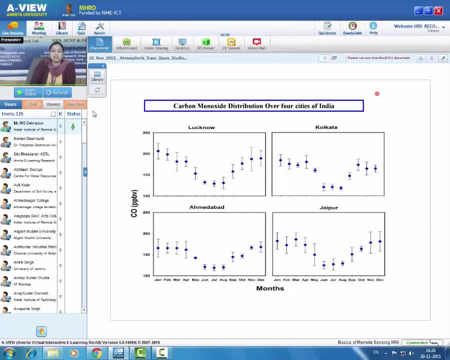 affect the distribution of these pollutants is atmospheric boundary layer. so atmospheric boundary layer depends on the heating of the surface. when the heating of surface is higher, the atmospheric boundary layer can go deeper in the atmosphere. during summer time, when- this time when sunlight is high, that time boundary layer can go deeper. 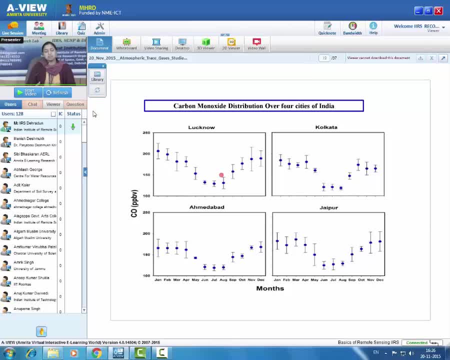 in the atmosphere and volume. the pollution which is emitted near the surface will get mixed up within the larger volume. however, during winter time boundary layer height is low and during that time the pollution is trapped in the lower volume. and when pollution is trapped in the lower volume, the 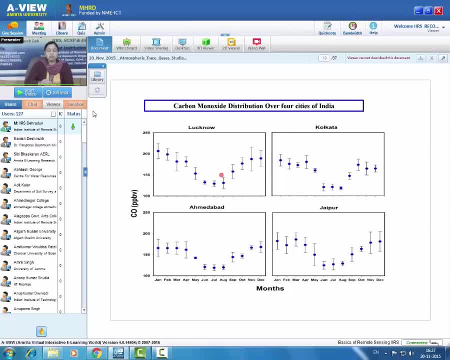 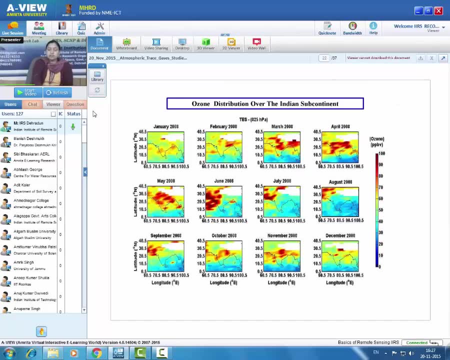 concentration of pollution will elevate because of these two processes. we are getting this type of monthly distribution. however, during winter time the pollution is trapped in the lower volume. the pollution is trapped in the lower volume. the pollution is trapped in the lower volume. however, we are getting different type of distribution for ozone. ozone does not show much high value during january and february. values are much higher during march, april, may and partially in june and after that, july, august and september values are low and again value picks the pollution and increases during october, november and december. then why this ozone is showing different feature? 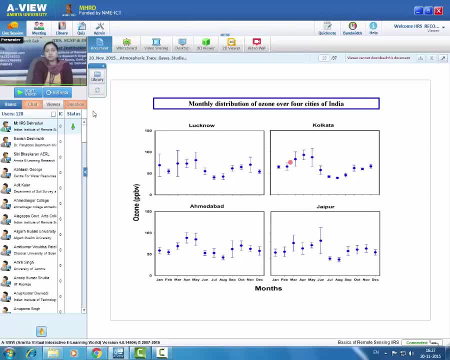 why this ozone is showing high values during march, april and may? because ozone is a secondary pollutant. it is dependent on the precursors, and though precursors are high during winter time- but sunlight is, sunlight intensity is not that high and ozone? ozone is produced through photochemistry, so when sufficient amount of pollution. 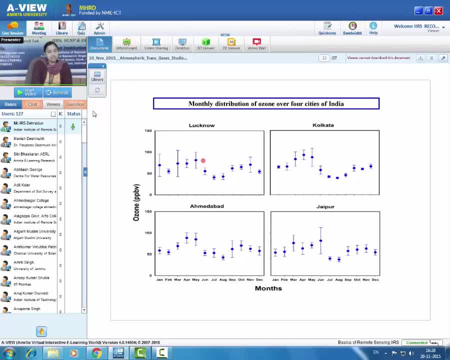 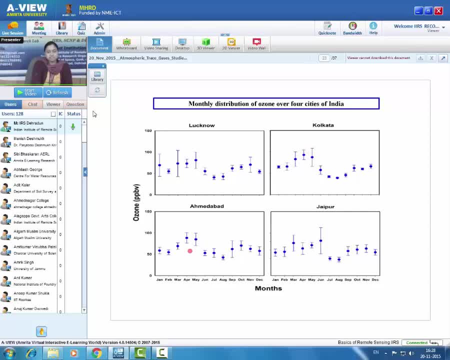 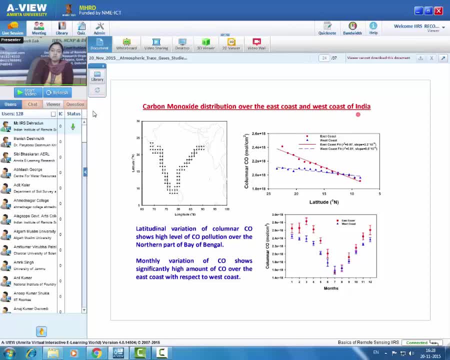 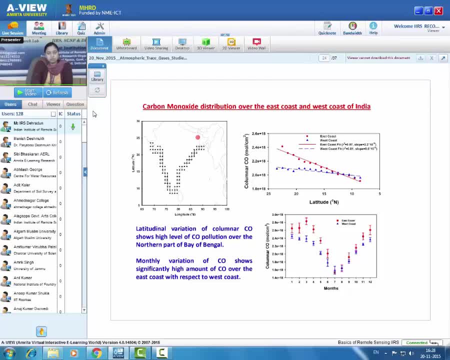 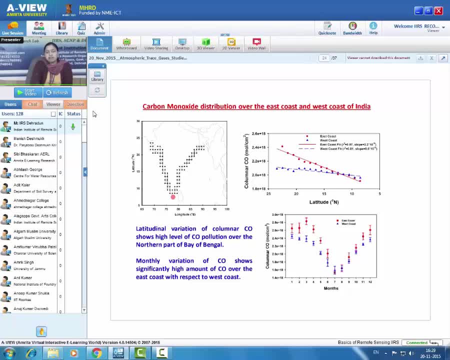 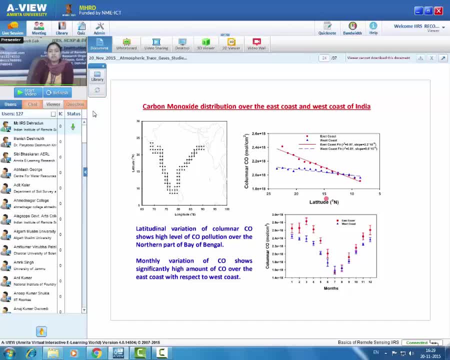 latitude and this clearly shows that for latitude less than 15 degree north, values are almost comparable across the India. however, there is a big difference between East Coast and West Coast when we see variation our per latitude more than 15 degree north. what is the reason? because high level of pollution is. 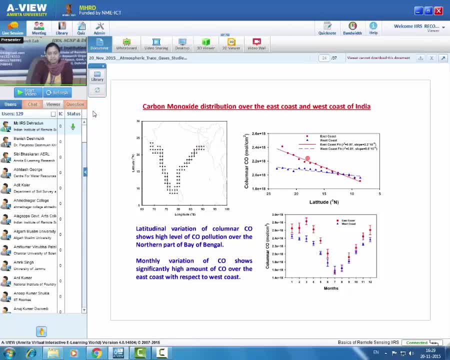 being injected from endo-gangetic plane. again to get information about the difference between the pollution over East Coast and West Coast, we have analyzed the monthly distribution of carbon monoxide over East Coast and West Coast and we have seen the difference is significant for each. region of India and we have seen the difference is significant for each region of India and we have seen the difference is significant for each region of India and we have seen the difference is significant for each month except during June, July, and month except during June, July and 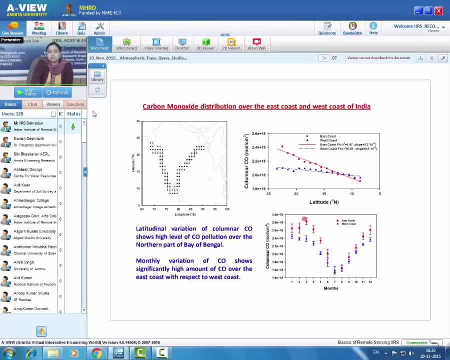 month, except during June, July and August, and difference is maximum during pre August and difference is maximum during pre August and difference is maximum during pre monsoon season during March, April and monsoon season during March April and monsoon season during March April and me. so this analysis shows that 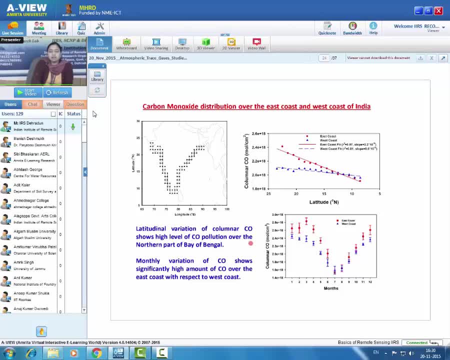 me. so this analysis shows that me. so this analysis shows that. latitudinal variation of columnar co. latitudinal variation of columnar co. latitudinal variation of columnar co. high value shows of carbon monoxide. high value shows of carbon monoxide. high value shows of carbon monoxide. pollution over the northern part of way. 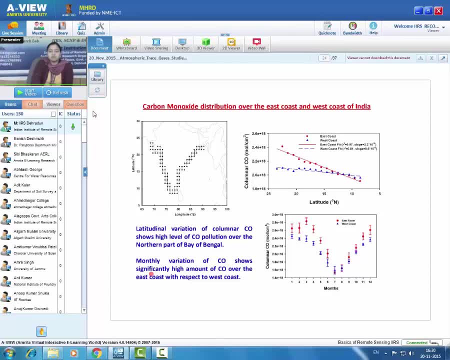 pollution over the northern part of way. pollution over the northern part of way of Bengal and monthly variation of co of Bengal and monthly variation of co of Bengal and monthly variation of co. shows significantly high amount of co. shows significantly high amount of co. shows significantly high amount of co over the East Coast with respect to West. 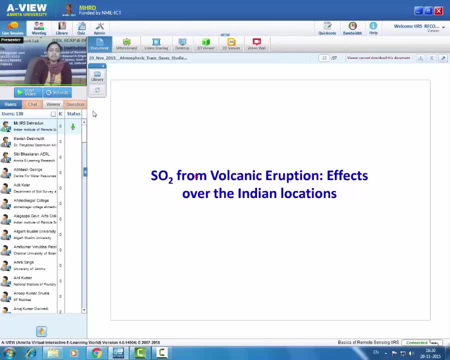 over the East Coast with respect to West. over the East Coast with respect to West Coast. satellite data can also help on Coast. satellite data can also help on Coast. satellite data can also help on the when we get high level of pollution, the when we get high level of pollution. 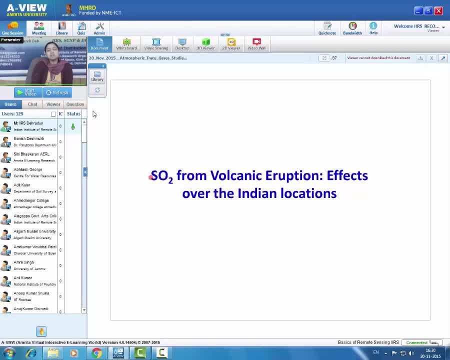 the when we get high level of pollution in the atmosphere and how that pollution in the atmosphere and how that pollution in the atmosphere and how that pollution plume is traveling from one location to plume is traveling from one location to plume is traveling from one location to other. so here is an example: sulfur. 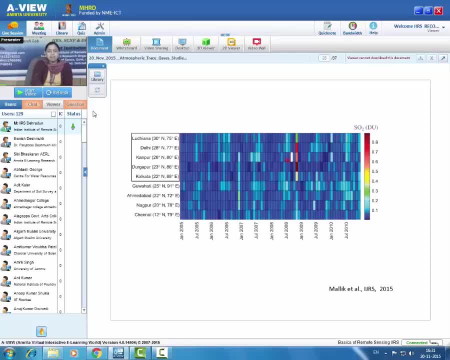 other. so here is an example sulfur other. so here is an example: sulfur dioxide: emission from volcanic eruption dioxide- emission from volcanic eruption dioxide. emission from volcanic eruption. in this plot, so total columnar sulfur in this plot, so total columnar sulfur. in this plot, so total columnar sulfur dioxide is shown and it is in Dobson. 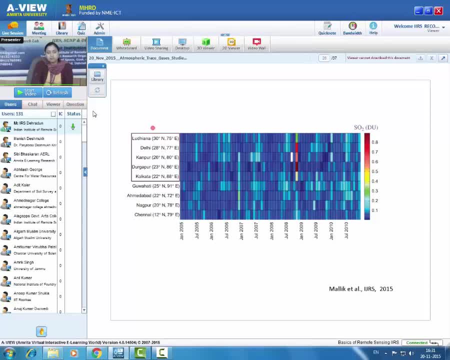 dioxide is shown and it is in Dobson dioxide is shown and it is in Dobson unit, and or it is analyzed over these unit, and or it is analyzed over these unit, and or it is analyzed over these locations: Ludhiana, Delhi, Kanpur. locations- Ludhiana, Delhi, Kanpur. 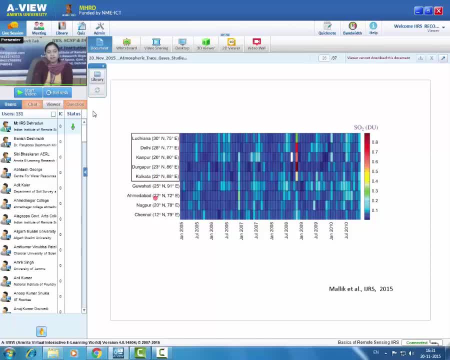 locations: Ludhiana, Delhi, Kanpur, Durga, poor Polkata, Guwahati, Ahmedabad, Durga, poor Polkata, Guwahati, Ahmedabad, Durga, poor Polkata, Guwahati, Ahmedabad, Nakpur and Chennai during January 2005. 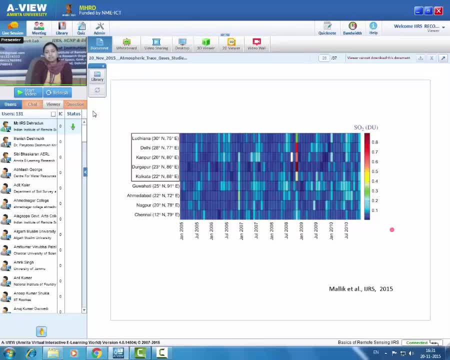 Nakpur and Chennai during January 2005. Nakpur and Chennai during January 2005 to December 2010. during these many years to December 2010, during these many years to December 2010, during these many years, this man, these many years we have seen. 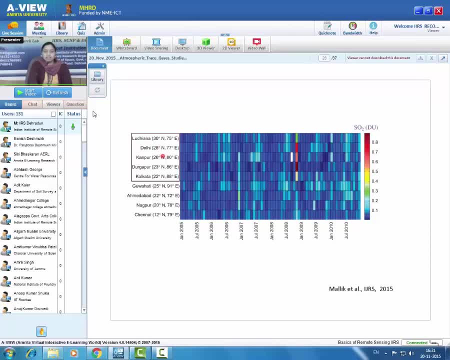 this man. these many years we have seen this man. these many years we have seen very high value over Ludhiana Delhi, very high value over Ludhiana Delhi, very high value over Ludhiana Delhi, Kanpur, Durga poor and Polkata during. Kanpur, Durga poor and Polkata during. 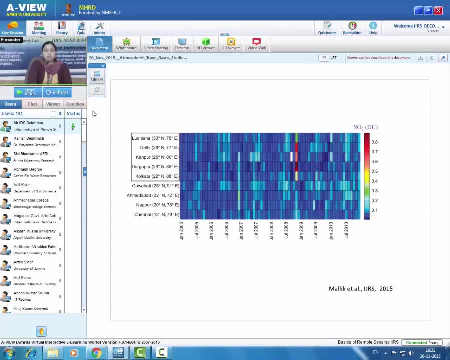 Kanpur, Durga poor and Polkata during November 2008. why we are getting very November 2008, why we are getting very November 2008, why we are getting very high value during this period. this we high value during this period, this we. 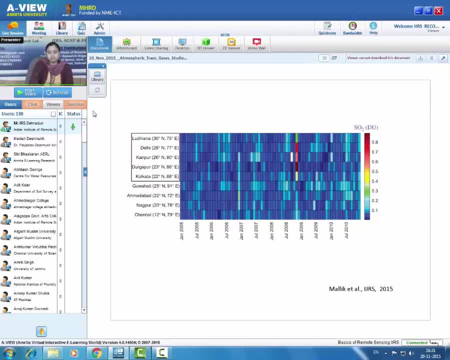 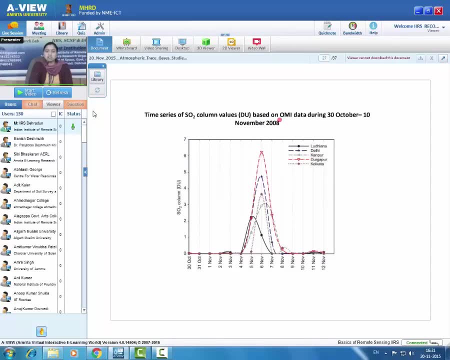 high value during this period. this we wanted to analyze. for this we have wanted to analyze. for this we have wanted to analyze. for this we have analyzed daily variation of sulfur: analyzed daily variation of sulfur. analyzed daily variation of sulfur dioxide column values you from the dioxide column values you from the. 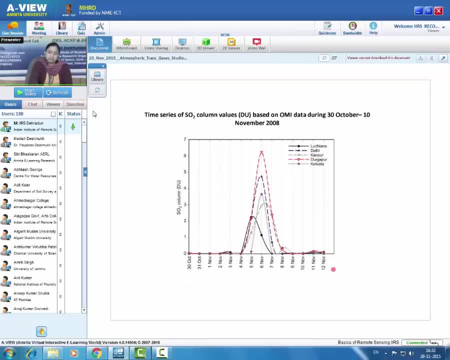 dioxide column values you from the home data during 30th of October to 12. home data during 30th of October to 12. home data during 30th of October to 12th of November. over these five locations of November. over these five locations. 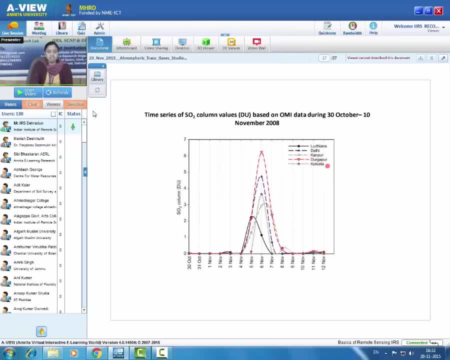 of November over these five locations where we have observed very high amount, where we have observed very high amount, where we have observed very high amount of sulfur dioxide during this particular of sulfur dioxide, during this particular of sulfur dioxide during this particular month, and we found that there was very 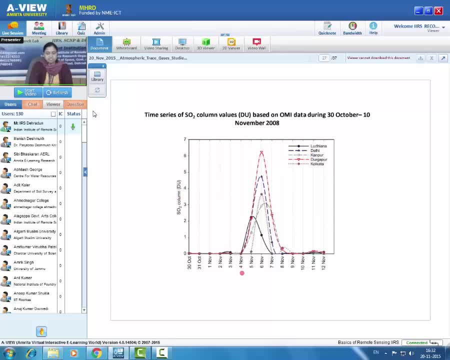 month and we found that there was very month and we found that there was very high amount of sulfur dioxide columnar high amount of sulfur dioxide columnar. high amount of sulfur dioxide columnar concentration during 4th of November to concentration during 4th of November to. 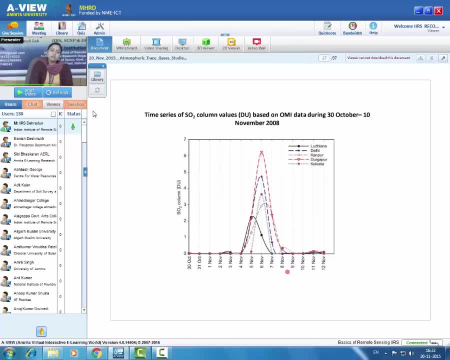 concentration during 4th of November to 8th of November. what was the reason of 8th of November? what was the reason of 8th of November? what was the reason of this very high, very, very high amount of this very high, very high amount of? 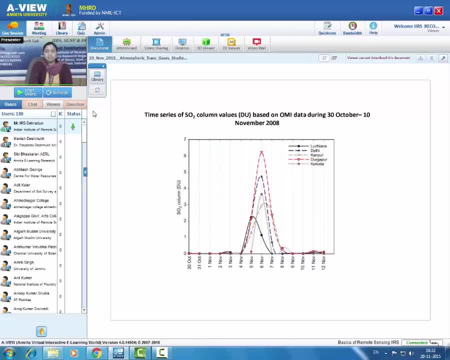 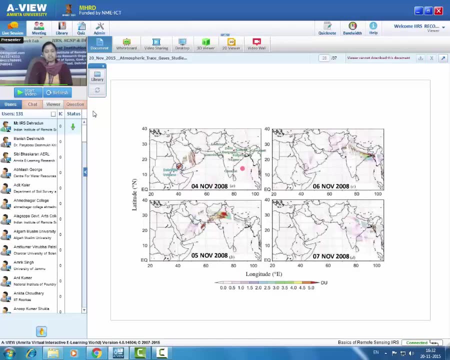 this very high, very high amount of sulfur dioxide. this we have sulfur dioxide. this we have sulfur dioxide. this we have investigated, when we have taken special investigated, when we have taken special investigated, when we have taken special distribution of sulfur dioxide for this. distribution of sulfur dioxide for this. 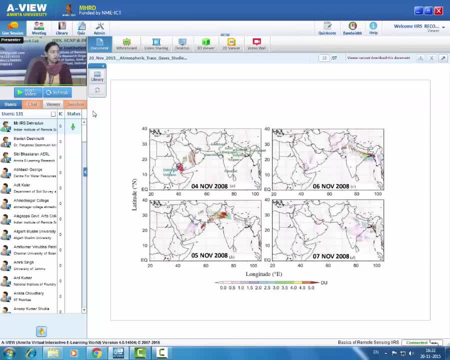 distribution of sulfur dioxide. for this you can see here in this plot one, you can see here in this plot one, you can see here in this plot one: volcanic eruption is occurring and volcanic eruption is occurring and volcanic eruption is occurring and because of that, a high plume of very 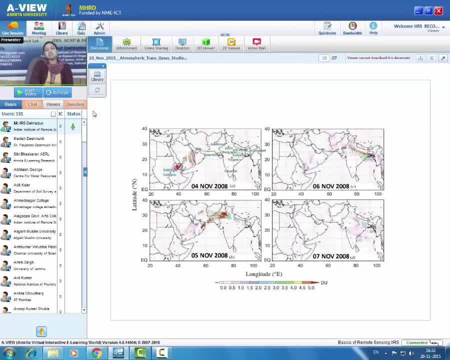 because of that, a high plume of very because of that, a high plume of very high intensity, very high concentration of high intensity, very high concentration of high intensity, very high concentration of sulfur dioxide is emerging at in started sulfur dioxide is emerging at in started sulfur dioxide is emerging at in started on 4th of November and this room 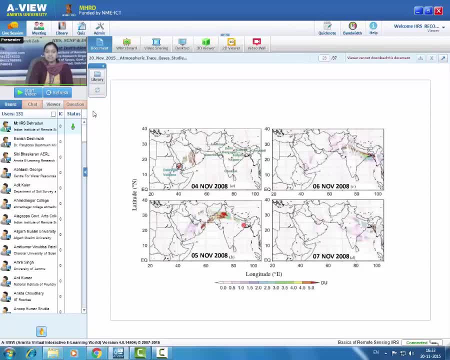 on 4th of November, and this room on 4th of November, and this room: eventually it got. eventually it got. eventually it got. transported to indo-gangetic plane on transported to indo-gangetic plane. on transported to indo-gangetic plane on 4th of November. this was the location of 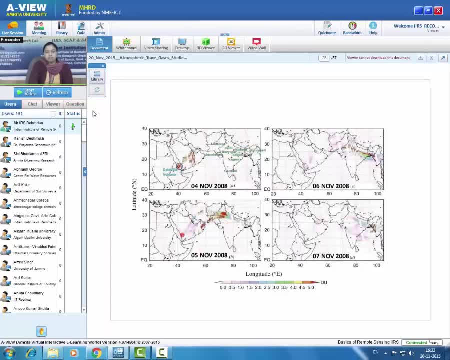 4th of November. this was the location of 4th of November. this was the location of plume on 5th of November. it transported plume on 5th of November. it transported plume on 5th of November. it transported by a Saudi Arabia and Iran towards the. 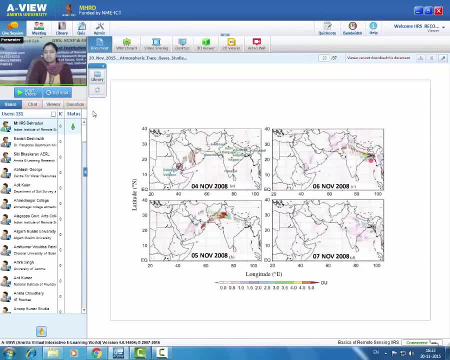 by a Saudi Arabia and Iran towards the. by a Saudi Arabia and Iran towards the indo-gangetic belt on 6th of November it. indo-gangetic belt on 6th of November. it. indo-gangetic belt on 6th of November: it is started dissipating. and 7th of 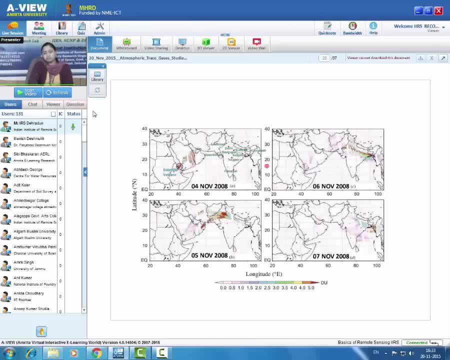 is started dissipating and 7th of is started dissipating and 7th of November. it is not near, it is not there. November. it is not near. it is not there. November. it is not near, it is not there. so this shows the distribution of any 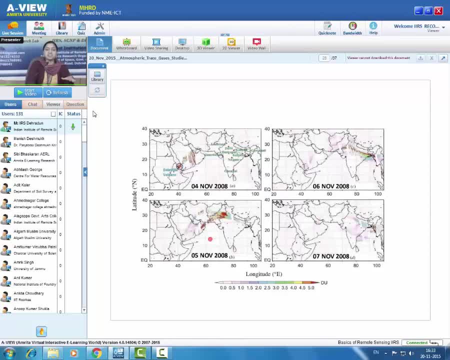 so this shows the distribution of any. so this shows the distribution of any pollution. if we see they analyze the pollution, if we see they analyze the pollution, if we see they analyze the spatial distribution of any pollution, we spatial distribution of any pollution, we spatial distribution of any pollution, we can identify the source, location of. 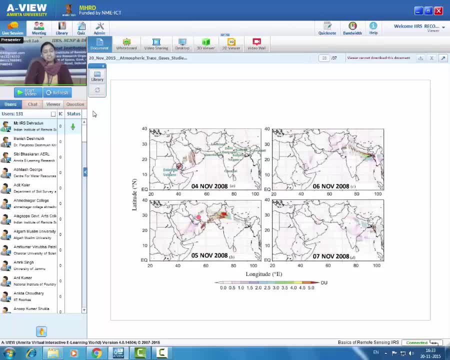 can identify the source location of, can identify the source location of high level of plumes and we can check the high level of plumes. and we can check the high level of plumes and we can check the pollution, how pollution emerged in pollution, how pollution emerged in. 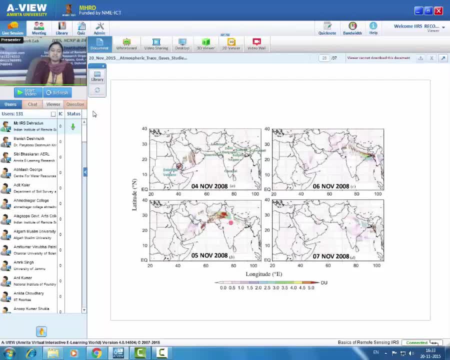 pollution, how pollution emerged in the atmosphere and how it got dissipated. the atmosphere and how it got dissipated. the atmosphere and how it got dissipated again. we study extreme co pollution again. we study extreme co pollution again. we study extreme co pollution episode due to forest. 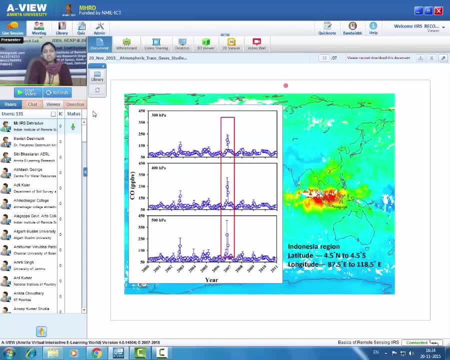 episode. due to forest episode. due to forest fire. for this one extreme co pollution fire. for this one extreme co pollution fire. for this one extreme co pollution event occurred over Indonesia during event occurred over Indonesia during. event occurred over Indonesia during September, November 2006. the background: 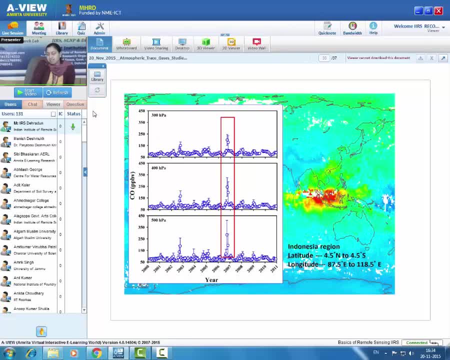 September, November 2006. the background- September November 2006. the background picture shows high level of carbon. picture shows high level of carbon. picture shows high level of carbon monoxide over this region. this is the monoxide over this region. this is the monoxide over this region. this is the Indonesian region. so, for the analysis of 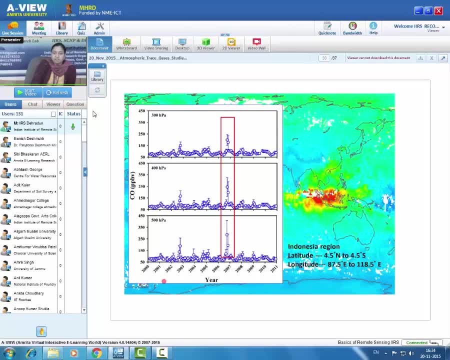 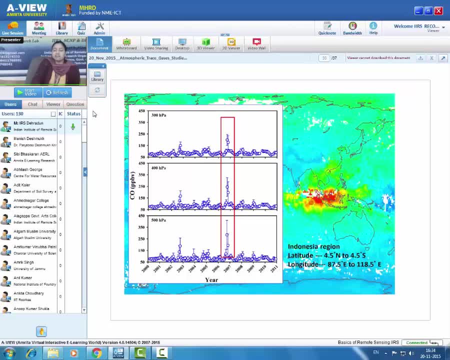 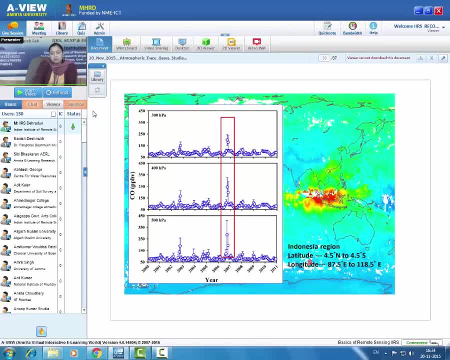 2010, we have taken a rectangular belt indoor over Indonesia, which is bounded indoor over Indonesia, which is bounded indoor over Indonesia, which is bounded by latitude: 4.5 degree north to 4.5. by latitude: 4.5 degree north to 4.5. 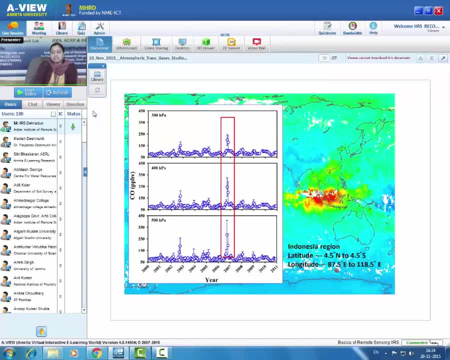 by latitude, 4.5 degree north to 4.5 degree south and longitude, 87.5 degree degree south and longitude 87.5 degree degree south and longitude 87.5 degree East, 218.5 degree East. so this is the. 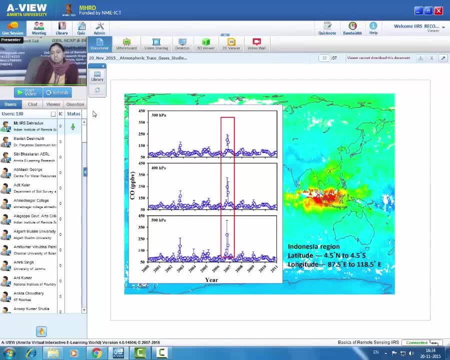 East 218.5 degree East. so this is the East 218.5 degree East. so this is the region which we have defined and we have region which we have defined and we have region which we have defined and we have taken average over this location for: 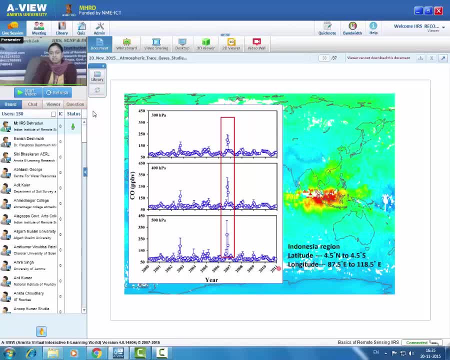 taken average over this location for: taken average over this location for every month since starting from 2000. every month since starting from 2000. every month since starting from 2000 to 2010. and we analyzed this data carbon to 2010. and we analyzed this data carbon. 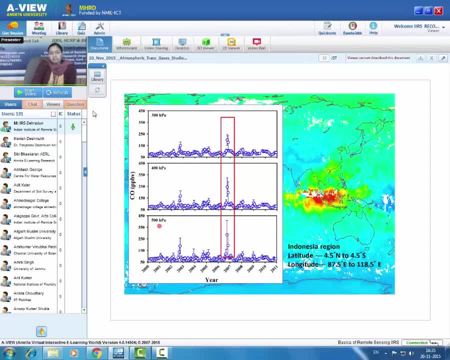 to 2010 and we analyzed this data. carbon monoxide data at pressure level: 500 monoxide data at pressure level- 500 monoxide data at pressure level: 500 hectopascal, 400 hectopascal and 300 hectopascal, 400 hectopascal and 300. 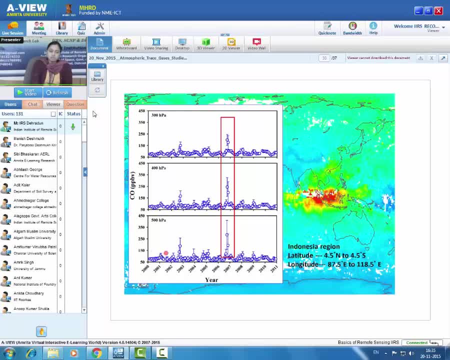 hectopascal, 400 hectopascal and 300 hecto Pascal. we have analyzed time hecto Pascal. we have analyzed time hecto Pascal. we have analyzed time series of this and we found that values series of this and we found that values series of this and we found that values are significantly very, very high during. 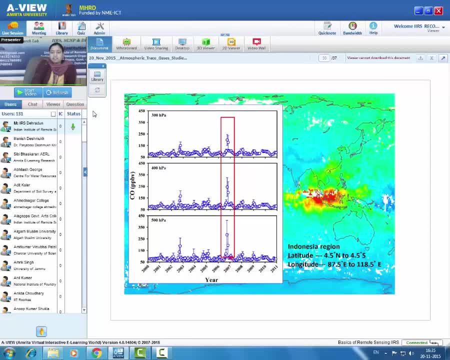 are significantly very, very high during are significantly very, very high during October November 2006. what is the reason October November 2006? what is the reason October November 2006? what is the reason? the- if you do see the values, it is more. the. if you do see the values, it is more. 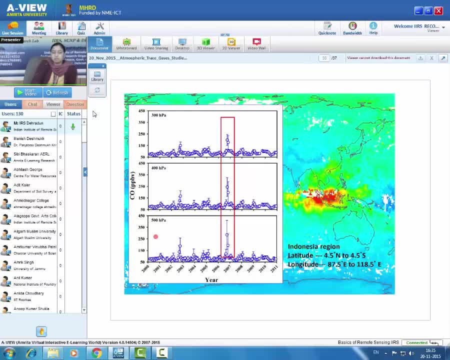 the. if you do see the values, it is more than 200 ppbv high, which is very, very than 200 ppbv high, which is very, very than 200 ppbv high, which is very, very large amount in the free troposphere. large amount in the free troposphere. 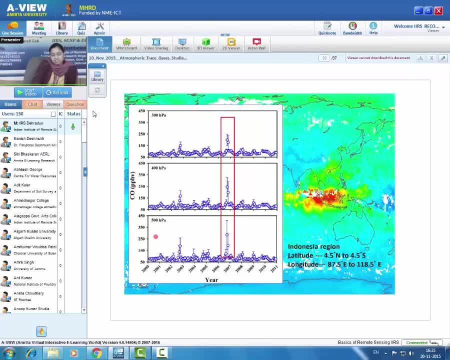 large amount in the free troposphere, where there is no source of carbon, where there is no source of carbon, where there is no source of carbon monoxide, so this is a very prominent monoxide. so this is a very prominent monoxide, so this is a very prominent event occurred, which is observed by 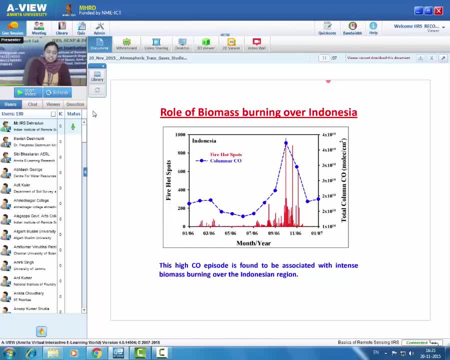 event occurred which is observed by event occurred which is observed by Muppet, so we tried to identify the Muppet. so we tried to identify the Muppet, so we tried to identify the source of this pollution, source of this source of this pollution, source of this source of this pollution, source of this pollution using fire, hot spots and total. 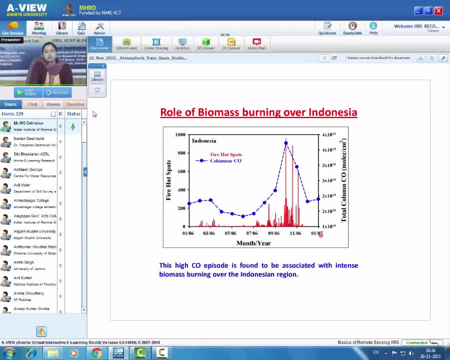 pollution using fire hot spots and total pollution using fire hot spots and total columnar content of co during 2006. so in columnar content of co during 2006. so in columnar content of co during 2006. so in this plot, month and year of this month. 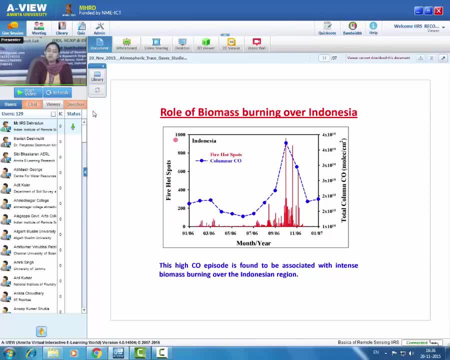 this plot: month and year of this month. this plot: month and year of this month and year is shown and x-axis and y-axis and year is shown and x-axis and y-axis and year is shown. and x-axis and y-axis shows fire hot spots, which is obtained. 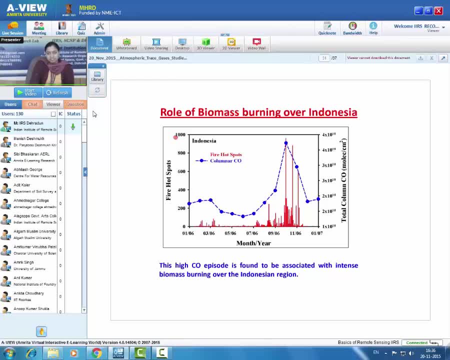 shows fire hot spots, which is obtained. shows fire hot spots, which is obtained from advanced alarm track scanning from advanced alarm track scanning from advanced alarm track scanning radiometer during that period on daily radiometer during that period, on daily radiometer during that period, on daily basis, and that are calculated over the 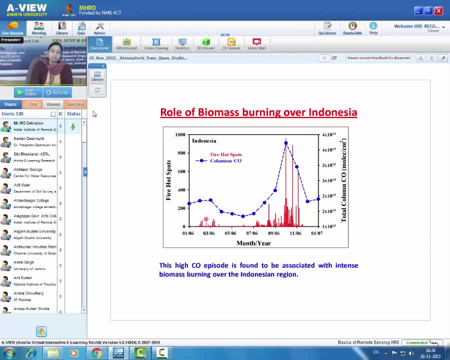 basis and that are calculated over the basis and that are calculated over the Indonesia region which we have defined, Indonesia region which we have defined, Indonesia region, which we have defined in the first side of this event, and we in the first side of this event, and we in the first side of this event, and we have plotted it with monthly average. 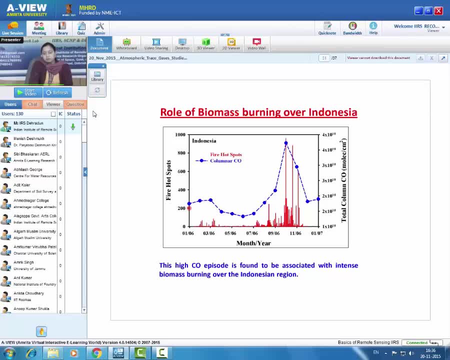 have plotted it with monthly average. have plotted it with monthly average, columnar co. if you view this plot, columnar co. if you view this plot, columnar co. if you view this plot closely, you will see that total column closely. you will see that total column closely. you will see that total column Narsu closely follows the variation of 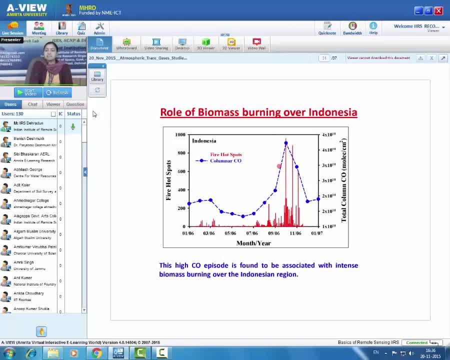 Narsu closely follows the variation of Narsu closely follows the variation of fire-hot spots and it elevate. it showed fire-hot spots and it elevate it showed fire-hot spots and it elevate. it showed elevated level during October and elevated level during October and elevated level during October and November when fire hot spot shows. 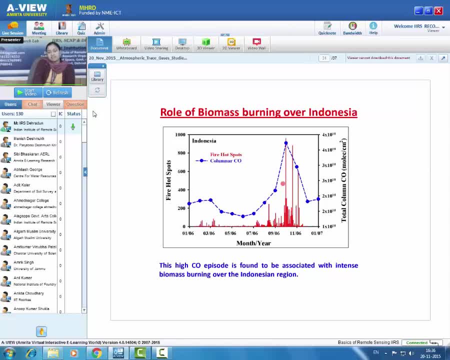 November, when fire hot spot shows. November, when fire hot spot shows maximum value, maximum value, maximum value. so from here we can suspect that this. so from here we can suspect that this. so from here we can suspect that this event was associated with biomass. event was associated with biomass. 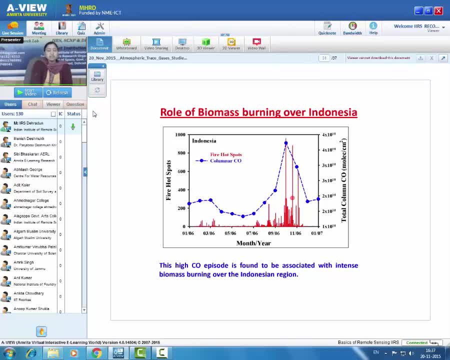 event was associated with biomass burning over Indonesia. but we can only burning over Indonesia, but we can only burning over Indonesia, but we can only suspect. can we say that exactly because suspect? can we say that exactly because suspect? can we say that exactly because of this only high level of pollution? 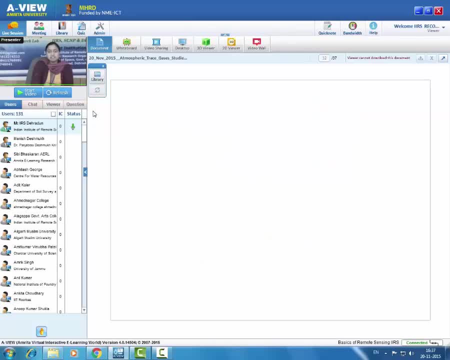 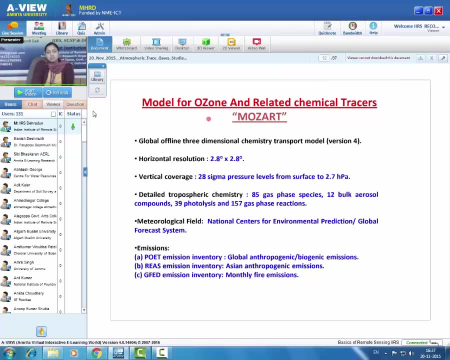 of this only high level of pollution, of this only high level of pollution, event occurred over Indonesia, yes, but event occurred over Indonesia, yes, but event occurred over Indonesia. yes, but not only using satellite data, but using- not only using satellite data, but using- not only using satellite data, but using chemistry transport model camera. we have 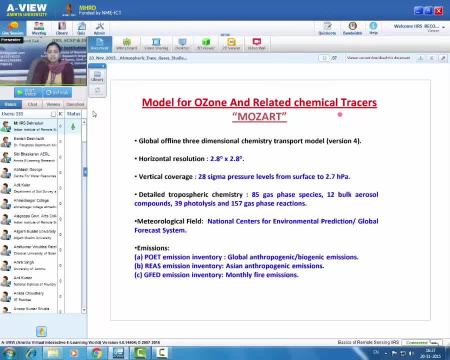 chemistry transport model camera. we have chemistry transport model camera. we have utilized model for ozone and related utilized model for ozone and related utilized model for ozone and related chemical tracers. Mozart: this is a global chemical tracers. Mozart: this is a global chemical tracers. Mozart: this is a global, offline three-dimensional chemistry. 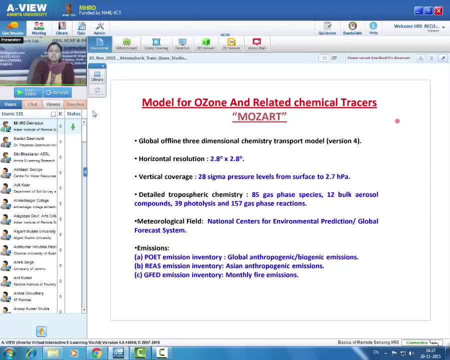 offline three-dimensional chemistry, offline three-dimensional chemistry, transport model, and we have utilized transport model and we have utilized transport model and we have utilized version 4 of this, this model, version 4 of this, this model, version 4 of this. this model mathematically computes the atmospheric. 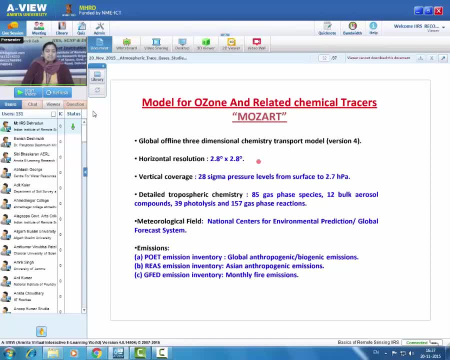 mathematically computes the atmospheric, mathematically computes the atmospheric chemistry and dynamics. for this, this chemistry and dynamics. for this, this chemistry and dynamics. for this, this model requires meteorological field and model requires meteorological field and model requires meteorological field and said data with logical field and emission. 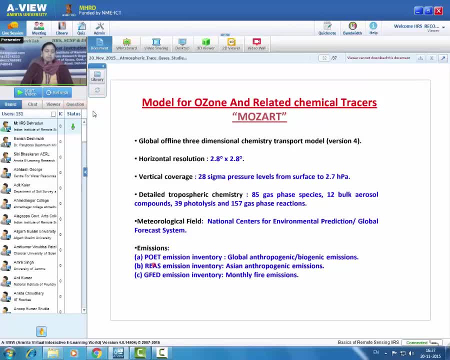 said data with logical field and emission said data with logical field and emission. emission of pollutants which are emission of pollutants, which are emission of pollutants which are taking participation in the photo. photo taking participation in the photo. photo taking participation in the photo. photo chemistry and chemistry of the. 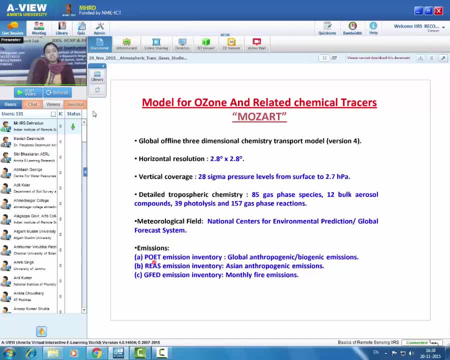 chemistry and chemistry of the chemistry and chemistry of the atmosphere. for that we have taken atmosphere, for that we have taken atmosphere, for that we have taken emission from emission inventories. these emission from emission inventories, these emission from emission inventories, these are poet emission inventory which gives. 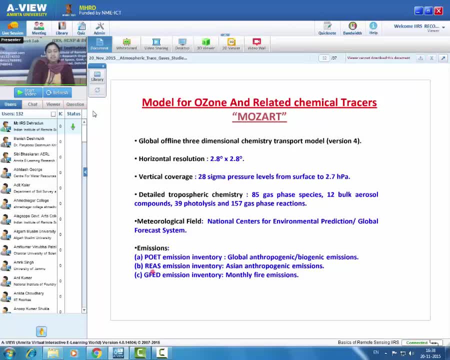 are poet emission inventory which gives are poet emission inventory. which gives the global anthropogenic and biogenic: the global anthropogenic and biogenic. the global anthropogenic and biogenic emissions, Riaz emission inventory. which emissions Riaz emission inventory. which emissions Riaz emission inventory. which gives the information about Asian. 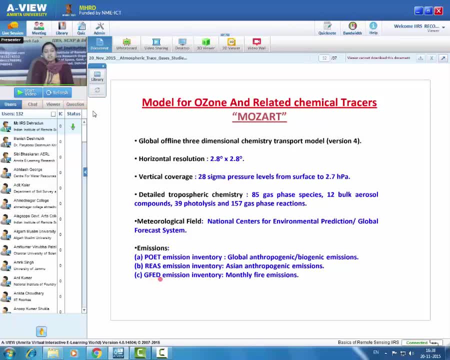 gives the information about Asian. gives the information about Asian anthropogenic emissions and global fire anthropogenic emissions and global fire. anthropogenic emissions and global fire emission database. gf-80 emission emission database. gf-80 emission emission database. gf-80 emission inventory, which gives the monthly fire. 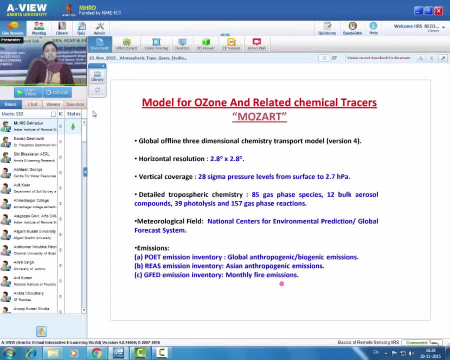 inventory which gives the monthly fire inventory, which gives the monthly fire emission all over the globe. so these emission all over the globe, so these emission all over the globe, so these emissions and meat logical data are emissions and meat logical data are emissions. and meat logical data are analyzed by this model, this model. 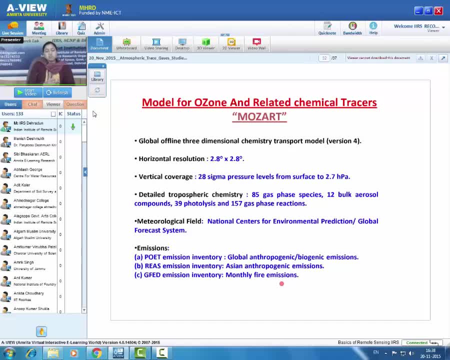 analyzed by this model. this model, analyzed by this model, this model mathematically computes how the mathematically computes, how the mathematically computes how the atmosphere is chemically. atmosphere is chemically, atmosphere is chemically evoluting. this is a. this model simulates 85. 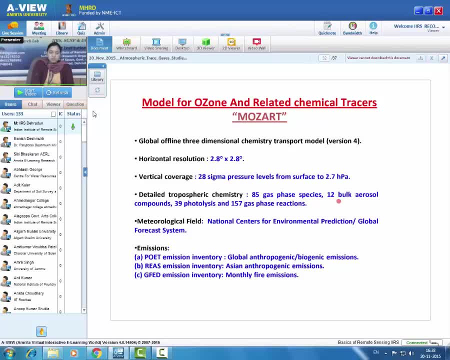 evoluting. this is a. this model simulates 85 evoluting. this is a. this model simulates 85 gas phase species, 12 bulk aerosol gas phase species, 12 bulk aerosol gas phase species, 12 bulk aerosol compounds, 39 photo lysis and 157 gas. 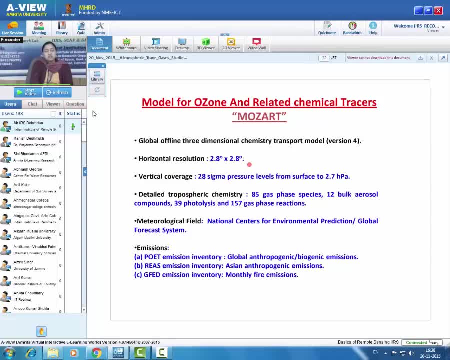 compounds: 39 photo lysis and 157 gas compounds: 39 photo lysis and 157 gas. phase reactions. the horizontal phase reactions: the horizontal phase reactions: the horizontal resolution of this model is poor, not resolution of this model is poor, not resolution of this model is poor, not where is good. because it is a global. 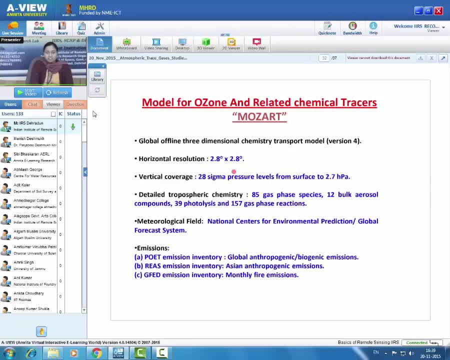 where is good because it is a global. where is good because it is a global model, so it is 2.8 cross 2.8 degree model. so it is 2.8 cross 2.8 degree model, so it is 2.8 cross 2.8 degree horizontal resolution and vertical. horizontal resolution and vertical horizontal resolution and vertical coverage from surface to around 2.7. coverage from surface to around 2.7. coverage from surface to around 2.7. hectopascal at 28 Sigma pressure levels. hectopascal at 28 Sigma pressure levels. 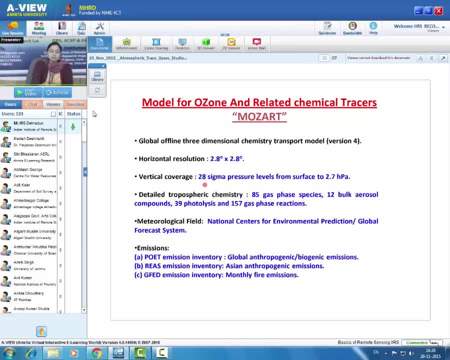 hectopascal at 28 Sigma pressure levels. this model calculates continuity. this model calculates continuity. this model calculates continuity equation for different gases. to see the equation for different gases. to see the equation for different gases. to see the evolution of that gas in the atmosphere. evolution of that gas in the atmosphere. 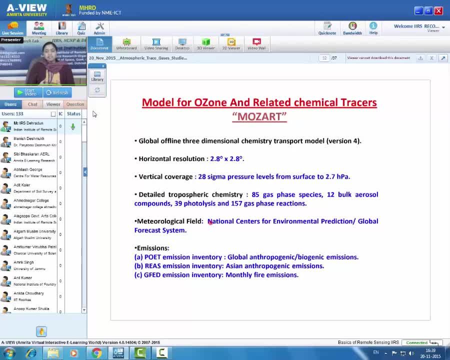 evolution of that gas in the atmosphere. as this model is mathematical model, it, as this model is mathematical model, it, as this model is mathematical model, it step-by-step calculates effect of step-by-step calculates effect of step-by-step. calculates effect of horizontal moment, effect of vertical. 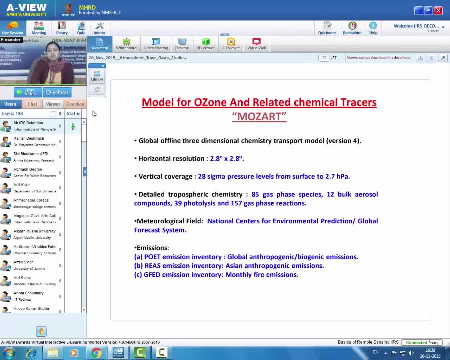 horizontal moment, effect of vertical horizontal moment, effect of vertical moment and effect of chemistry. so we have moment and effect of chemistry, so we have moment and effect of chemistry. so we have utilized this model with this emission, utilized this model with this emission, utilized this model with this emission, inventory and meteorological data, and we 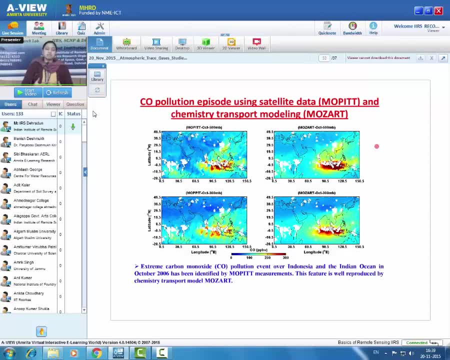 inventory and meteorological data and we inventory and meteorological data and we have tried to simulate the same feature, have tried to simulate the same feature, have tried to simulate the same feature- same atmospheric phenomenon, which is same atmospheric phenomenon, which is same atmospheric phenomenon which is happening in real. so this figure shows: 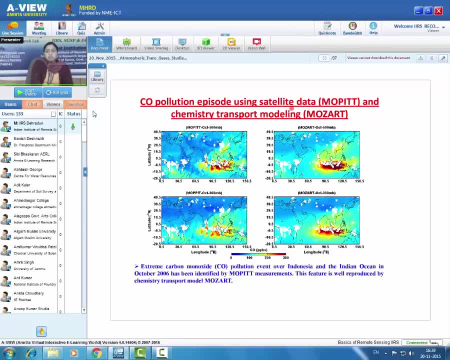 happening in real. so this figure shows happening in real. so this figure shows carbon monoxide pollution episode using carbon monoxide pollution episode using carbon monoxide pollution episode using satellite data: Muppet and chemistry satellite data. Muppet and chemistry satellite data. Muppet and chemistry transport modeling. Mozart, so left-hand. 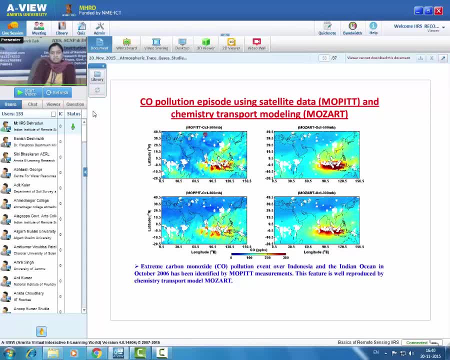 transport modeling Mozart. so left-hand transport modeling Mozart. so left-hand side figure shows Muppet distribution. side figure shows Muppet distribution. side figure shows Muppet distribution. measurement of pollution. in the measurement of pollution. in the measurement of pollution in the troposphere during October 2006 at 500. 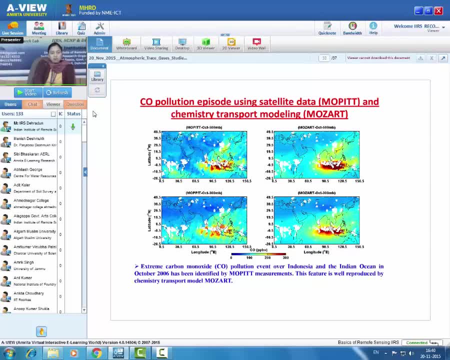 troposphere during October 2006 at 500. troposphere during October 2006 at 500. hectopascal or millibar and rather down hectopascal or millibar and rather down. hectopascal or millibar and rather down. her in downside figure shows Muppet. 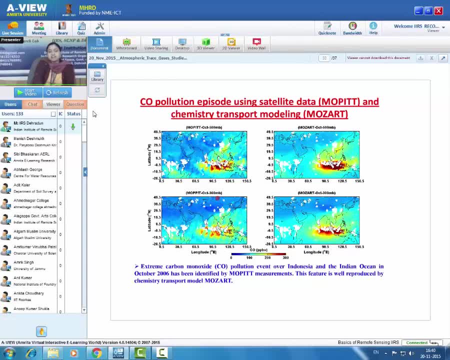 her in downside figure shows Muppet. her in downside figure shows Muppet. measurement for October 2006 at 300. measurement for October 2006 at 300. measurement for October 2006 at 300. millibar. right-hand side figure shows the millibar right-hand side figure shows the. 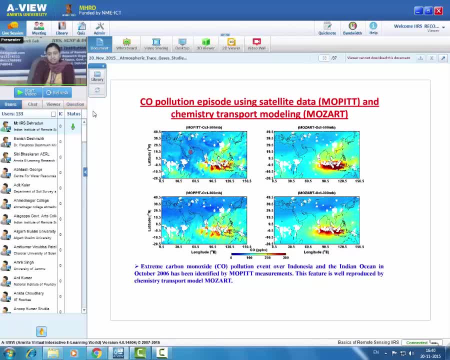 millibar right-hand side figure shows the same thing, but simulated by Mozart. this same thing, but simulated by Mozart. this same thing, but simulated by Mozart. this is real-time observation. this is is real-time observation. this is is real-time observation. this is calculated by model, and this model is. 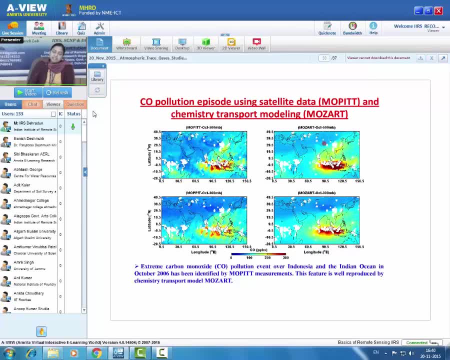 calculated by model, and this model is calculated by model and this model is simulating atmospheric chemistry by simulating atmospheric chemistry, by simulating atmospheric chemistry, by taking emission inventories as well as taking emission inventories, as well as taking emission inventories as well as mythology, so extremes, carbon monoxide. 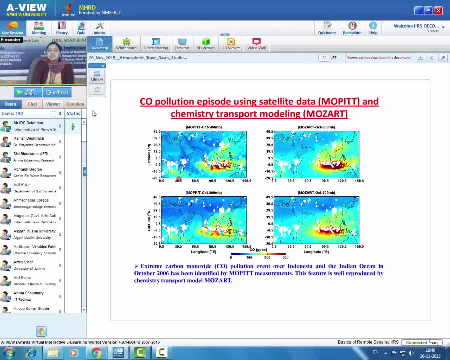 mythology: so extremes carbon monoxide mythology, so extremes carbon monoxide pollution. plume event occurred over pollution. plume event occurred over pollution. plume event occurred over Indonesia. is very well reproduced by Indonesia. is very well reproduced by Indonesia. is very well reproduced by chemistry. transport model: Mozart can see: 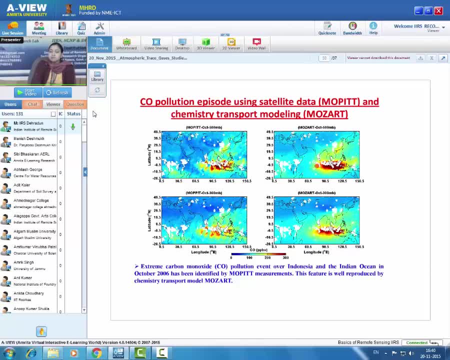 chemistry transport model. Mozart can see chemistry transport model. Mozart can see that values are high over this region, that values are high over this region, that values are high over this region. this is also reproduced by our model for this is also reproduced by our model, for this is also reproduced by our model for both the pressure levels. this indicates: 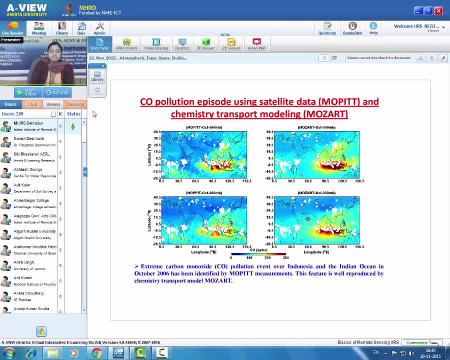 both the pressure levels. this indicates both the pressure levels. this indicates that our model can be taken as that. our model can be taken as that. our model can be taken as reliable. yes, our model is considering reliable. yes, our model is considering reliable. yes, our model is considering everything correctly. it is take, it has. 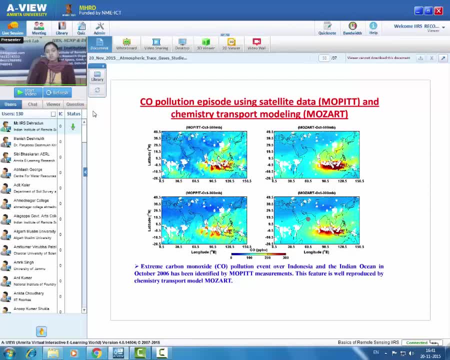 everything correctly, it is take. it has everything correctly, it is take. it has taken correct emissions. it has simulated, taken correct emissions. it has simulated, taken correct emissions. it has simulated the atmospheric chemistry correctly, so we the atmospheric chemistry correctly, so we the atmospheric chemistry correctly, so we can rely on our model. then we can. 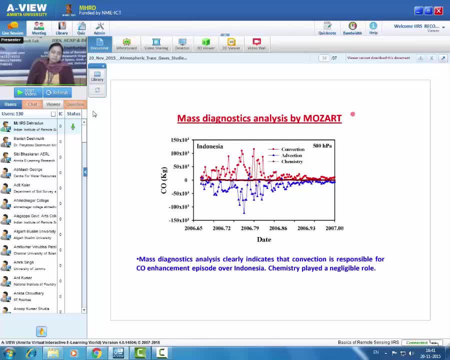 can rely on our model, then we can can rely on our model, then we can define: because my model is a mathematical define, because my model is a mathematical define, because my model is a mathematical simulation, we can take information, we can simulation. we can take information, we can. 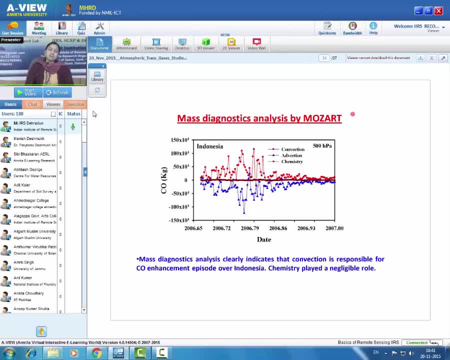 simulation. we can take information, we can take out other information from model, take out other information from model, take out other information from model which we cannot take out from the, which we cannot take out from the, which we cannot take out from the satellite data. what are these additional? 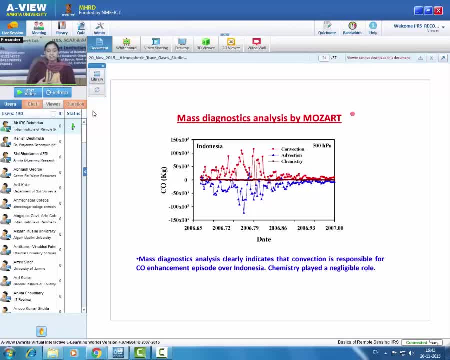 satellite data. what are these additional satellite data? what are these additional information, these additional information, these additional information, these additional informations are effect of different informations, are effect of different informations, are effect of different atmospheric processes, like satellite atmospheric processes, like satellite atmospheric processes, like satellite data will tell you that this is the 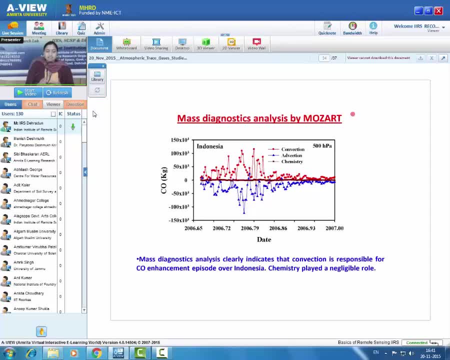 data will tell you that this is the data will tell you that this is the pollution distribution over this location. pollution distribution over this location. pollution distribution over this location: this is a dead satellite attack and give this is a dead satellite attack and give this is a dead satellite attack and give information that suddenly, over this, 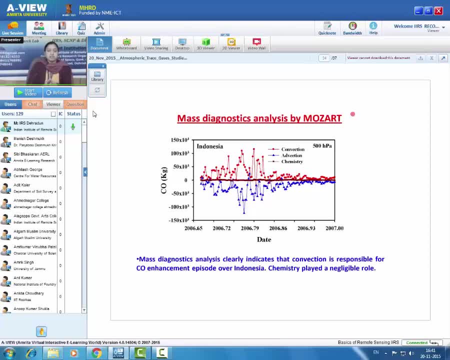 information that suddenly, over this information, that suddenly over this region, we have received very high amount region. we have received very high amount region. we have received very high amount of pollution. but satellite data will not of pollution, but satellite data will not of pollution, but satellite data will not tell any information about the specific 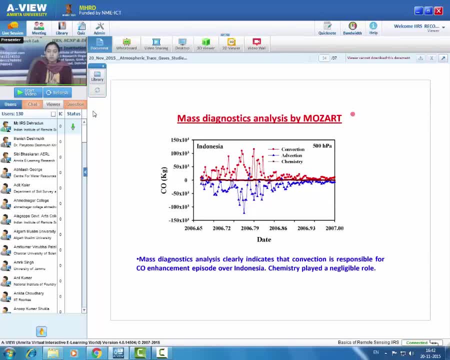 tell any information about the specific. tell any information about the specific source and amount of contribution coming source and amount of contribution coming source and amount of contribution coming from that source and what is the from that source and what is the from that source and what is the contribution from different atmospheric. 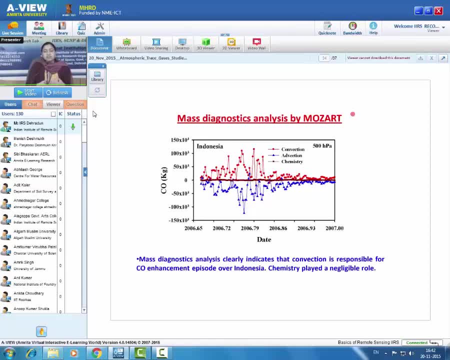 contribution from different atmospheric contribution from different atmospheric processes. but model is simulating processes, but model is simulating processes. but model is simulating everything mathematically, so it is taking everything mathematically. so it is taking everything mathematically, so it is taking effect of horizontal motion. again it is. 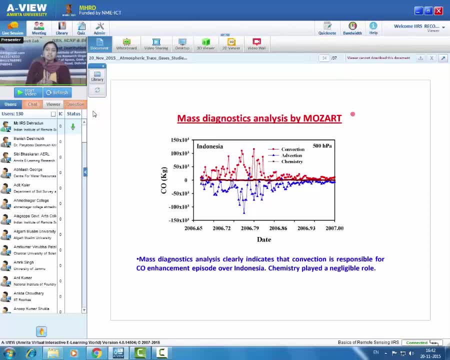 effect of horizontal motion. again it is effect of horizontal motion, again it is carried out, calculating effect of vertical. carried out, calculating effect of vertical carried out, calculating effect of vertical motion. again it is calculating effect of motion. again it is calculating effect of motion. again it is calculating effect of transformation of chemical species. and then it 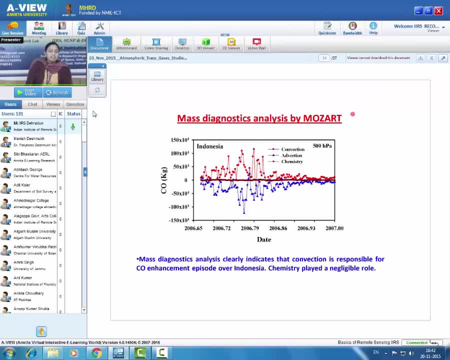 transformation of chemical species, and then it transformation of chemical species and then it is simulating atmosphere, then this model is simulating atmosphere, then this model is simulating atmosphere. then this model can give you information about the, can give you information about the, can give you information about the different processes and it can give you. 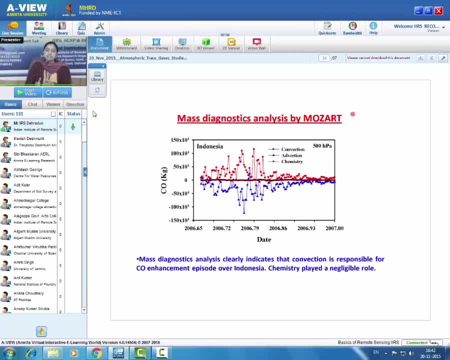 different processes and it can give you different processes and it can give you information that how much of pollution, information that, how much of pollution, information that how much of pollution is being added with or removed by, is being added with or removed by, is being added with or removed by different atmospheric processes. so for 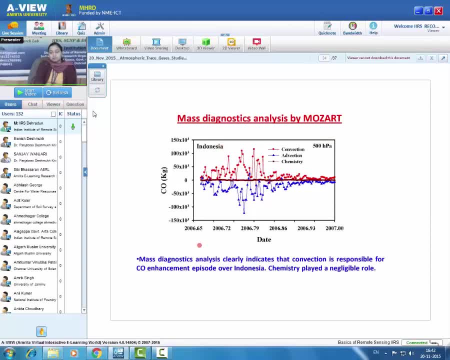 different atmospheric processes, so for different atmospheric processes. so for this we have taken mass diagnostic. this we have taken mass diagnostic. this we have taken mass diagnostic analysis of model and x-axis shows date analysis of model and x-axis shows date analysis of model and x-axis shows date and it varies from September 2006 to. 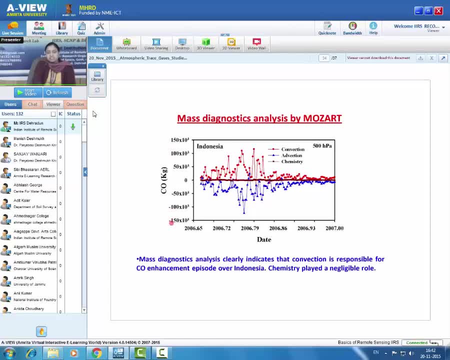 and it varies from December 2006 to. and it varies from December 2006 to December 2006. and y-axis show carbon December 2006. and y-axis show carbon December 2006. and y-axis show carbon monoxide, but weight which is introduced. 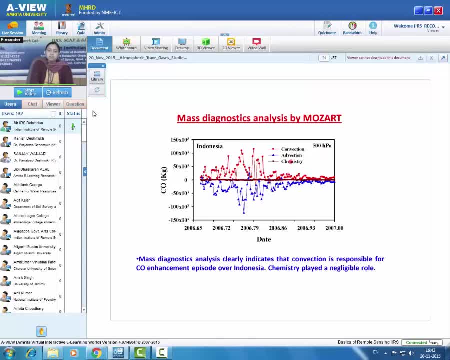 monoxide but weight which is introduced. monoxide but weight which is introduced at 500 hectare Pascal, because of at 500 hectare Pascal, because of at 500 hectare Pascal, because of convection, advection and chemistry it, convection, advection and chemistry it. 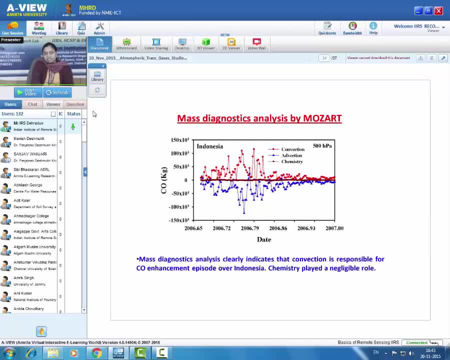 convection, advection and chemistry. it shows that over Indonesia region, here I shows that over Indonesia region, here I shows that over Indonesia region, here I would like to remind that Indonesia would like to remind that Indonesia would like to remind that Indonesia region is average region, which we have. 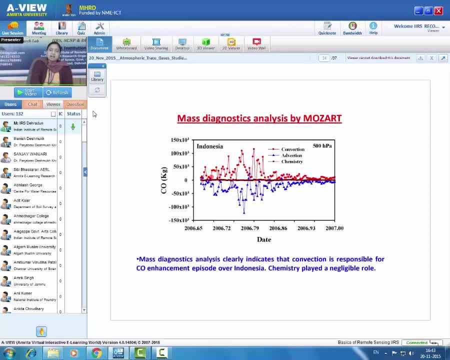 region is average region which we have. region is average region which we have defined in first sight over that region, defined in first sight over that region, defined in first sight over that region. how the effect of convection is varying. how the effect of convection is varying. 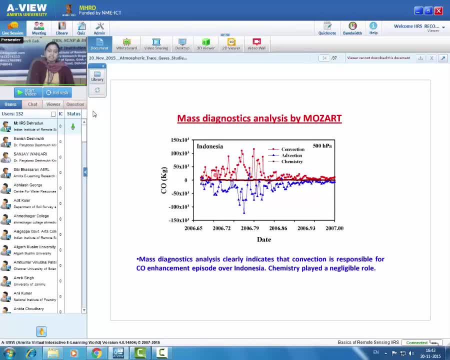 how the effect of convection is varying. so it is showing that, because of so, it is showing that, because of so, it is showing that because of convection, this red- red color variation, convection, this red- red color variation, convection, this red- red color variation, shows the effect of convection and it 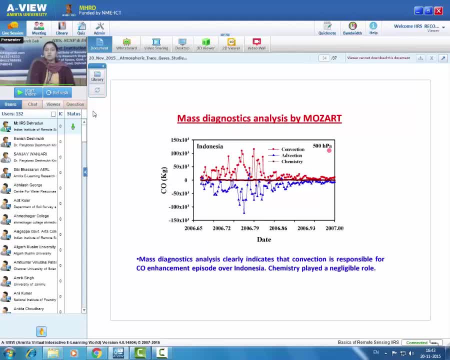 shows the effect of convection and it shows the effect of convection and it shows that carbon monoxide is, shows that carbon monoxide is, shows that carbon monoxide is enhancing over 500 hectare Pascal. because enhancing over 500 hectare Pascal, because enhancing over 500 hectare Pascal because of convection, the contribution of 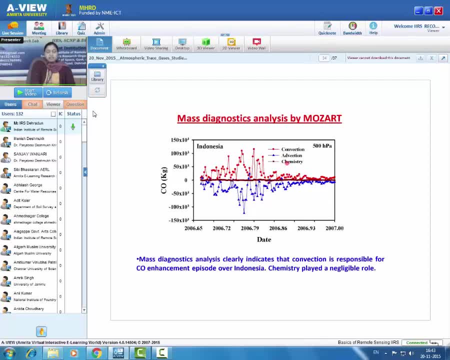 of convection, the contribution of of convection. the contribution of convection is positive. whereas convection is positive. whereas convection is positive. whereas contribution of advection is shown. contribution of advection is shown. contribution of advection is shown negative. so this indicates that, because of 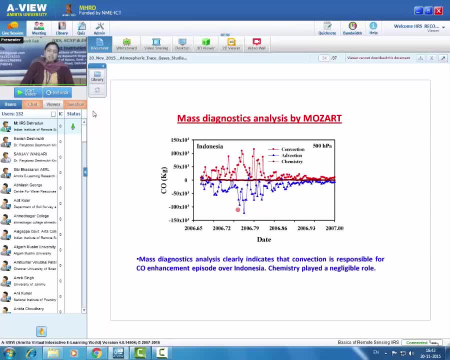 negative. so this indicates that because of negative. so this indicates that because of convection process: the high the carbon convection process, the high the carbon convection process, the high the carbon monoxide is increasing over 500 hectare. monoxide is increasing over 500 hectare. 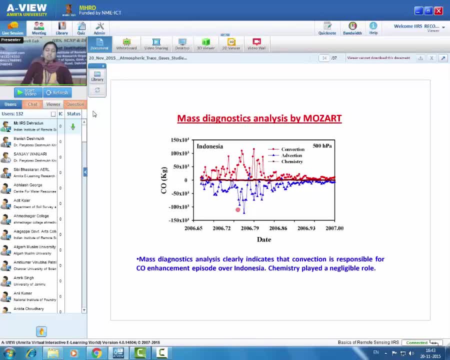 monoxide is increasing over 500 hectare Pascal, whereas because of advection Pascal, whereas because of advection Pascal, whereas because of advection process, the amount of carbon monoxide is process, the amount of carbon monoxide is process, the amount of carbon monoxide is decreasing over this region. this 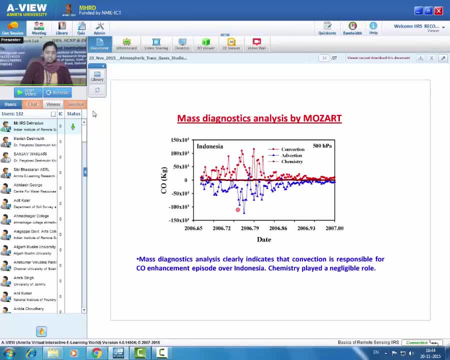 decreasing over this region. this decreasing over this region. this indicates that near surface and enhanced indicates that near surface and enhanced indicates that near surface and enhanced, this biomass burning event occurred and this biomass burning event occurred. and this biomass burning event occurred and because of conviction, this event, this 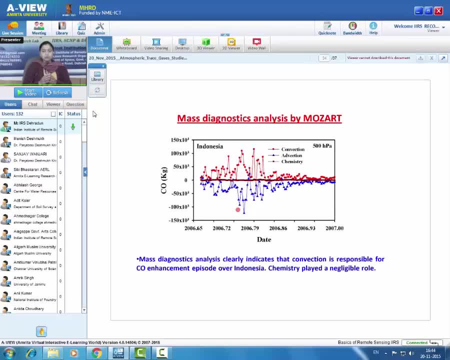 because of conviction, this event, this because of conviction, this event, this emission got transported over high altitude. emission got transported over high altitude emission got transported over high altitude at 500 hectare Pascal and over that at 500 hectare Pascal and over that at 500 hectare Pascal and over that region, advection started occurring and 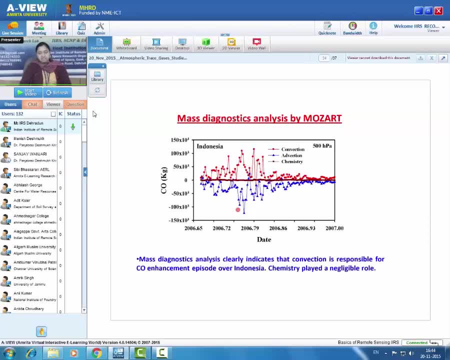 region advection started occurring, and region advection started occurring and because of that the pollution plume got. because of that the pollution plume got. because of that the pollution plume got dissipated slowly with time. and here dissipated slowly with time and here dissipated slowly with time. and here again an additional information is also. 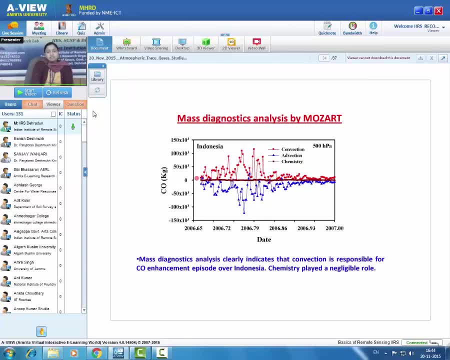 again, an additional information is also again, an additional information is also introduced. that is chemistry. if you see introduced, that is chemistry. if you see introduced, that is chemistry. if you see, contribution of chemistry is almost, contribution of chemistry is almost, contribution of chemistry is almost negligible, it is always zero. this means 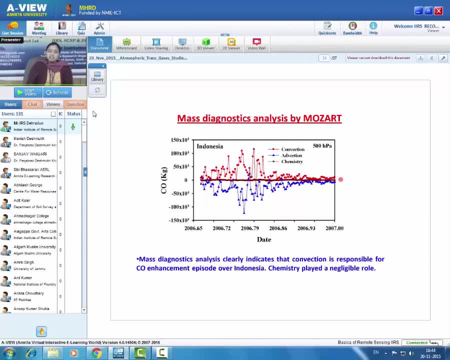 negligible. it is always zero. this means negligible, it is always zero. this means chemistry is not occurring at this, chemistry is not occurring at this, chemistry is not occurring at this role for this distribution. so this is a role for this distribution, so this is a role for this distribution. so this is a very important information which is 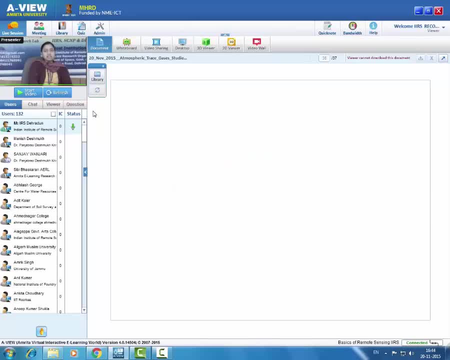 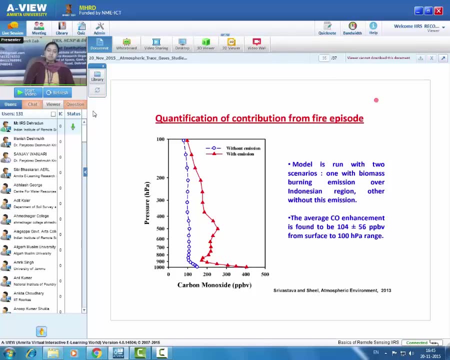 very important information, which is very important, information which is given by our model which cannot be taken, given by our model, which cannot be taken, given by our model, which cannot be taken from the satellite data. again, I told you from the satellite data. again I told you from the satellite data. again I told you that the model simulation is mathematical. 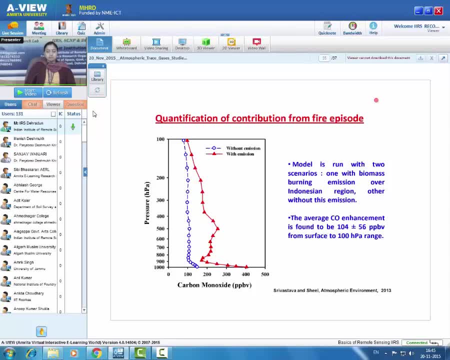 that the model simulation is mathematical, that the model simulation is mathematical simulation and it takes the emission simulation and it takes the emission simulation and it takes the emission inventories into picture. it takes the inventories into picture. it takes the inventories into picture. it takes the emission near the surface, it takes the. 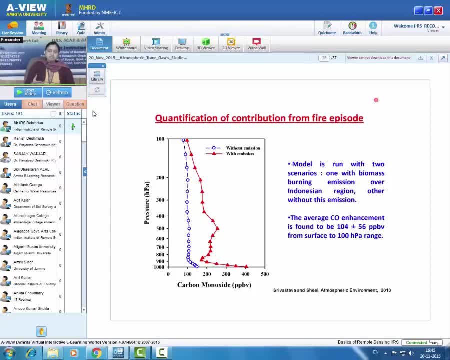 emission near the surface. it takes the emission near the surface, it takes the mythology also and it allows the mythology also, and it allows the mythology also and it allows the atmosphere to change from its initial atmosphere, to change from its initial atmosphere, to change from its initial condition. in this process, as we are, 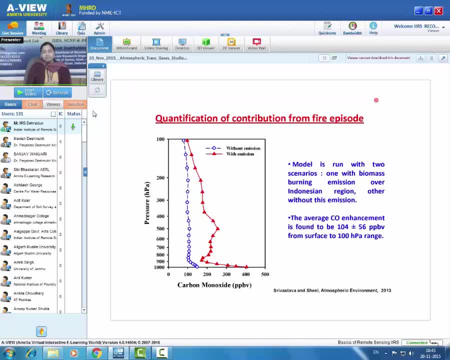 condition in this process, as we are condition in this process, as we are giving emissions separately, we can they giving emissions separately. we can they giving emissions separately, we can. they are. we can take out the emission from are. we can take out the emission from are. we can take out the emission from this and we can also see if there is no. 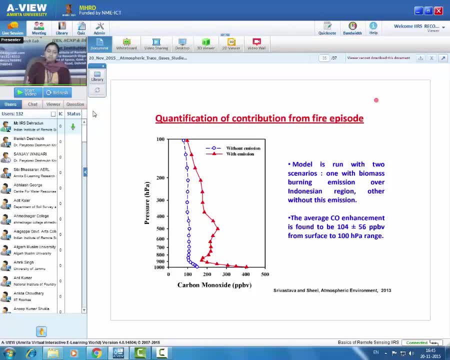 this and we can also see if there is no this and we can also see, if there is no emission, how the a particular pollution emission, how the a particular pollution emission, how the a particular pollution, will vary in the atmosphere, so we have. will vary in the atmosphere, so we have. 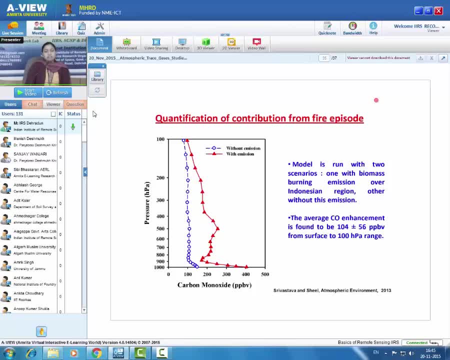 will vary in the atmosphere. so we have run this model in two scenarios: one with. run this model in two scenarios: one with. run this model in two scenarios: one with emission and second without emission in emission and second without emission in emission and second without emission. in first process we have switched off. 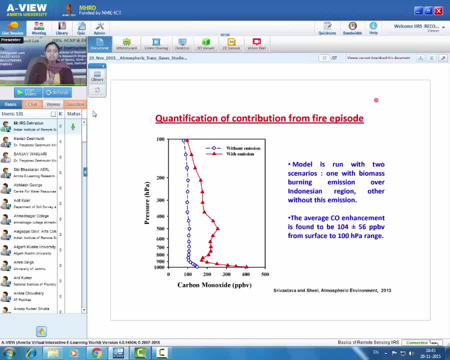 first process we have switched off. first process we have switched off emission and we have taken normal run and emission and we have taken normal run and emission and we have taken normal run. and in second process we have switched. in second process we have switched. in second process we have switched off emission over this particular region. 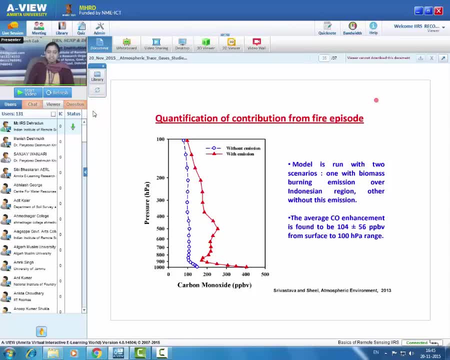 off emission over this particular region. off emission over this particular region. only emission because of biomass burning, only emission because of biomass burning, only emission because of biomass burning. and we allowed our model to evolute in and we allowed our model to evolute in and we allowed our model to evolute in the atmosphere. and it should start from. 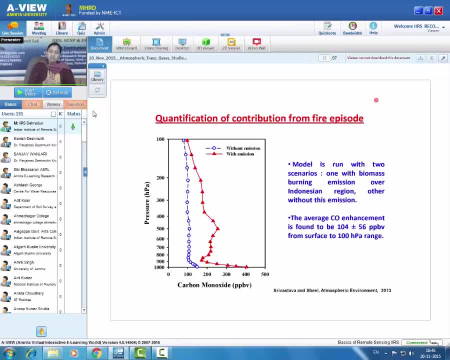 the atmosphere, and it should start from the atmosphere, and it should start from the beginning, and it should take consider the beginning, and it should take, consider the beginning, and it should take consider all the atmospheric phenomenon, all the, all the atmospheric phenomenon, all the, all the atmospheric phenomenon, all the emission, but without biomass burning. 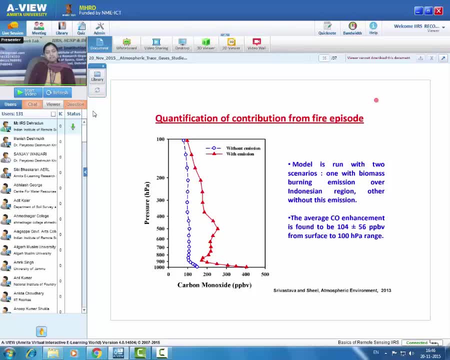 emission, but without biomass burning. emission, but without biomass burning, which occurred over Indonesia, then we which occurred over Indonesia, then we which occurred over Indonesia, then we have two graphs, one is the vertical. have two graphs, one is the vertical. have two graphs. one is the vertical: distribution of carbon monoxide. these 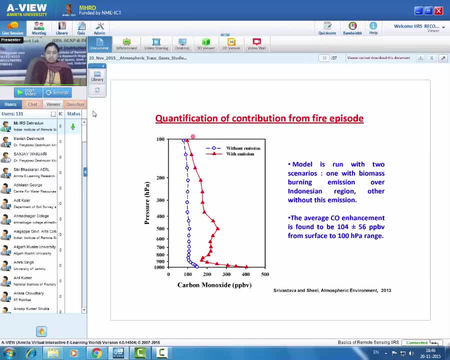 distribution of carbon monoxide, these distribution of carbon monoxide, these red curves over the over this Indonesia. red curves over the over this Indonesia, red curves over the over this Indonesia region. and one without emission when region and one without emission when region and one without emission when there is no emission. what would have been? 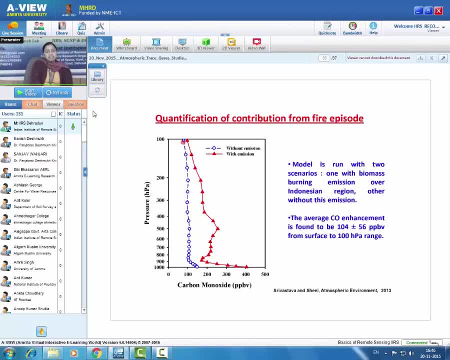 there is no emission. what would have been? there is no emission. what would have been the vertical distribution of carbon? the vertical distribution of carbon, the vertical distribution of carbon monoxide. that is also simulated by this monoxide. that is also simulated by this monoxide. that is also simulated by this model. so, model run with two scenario one: 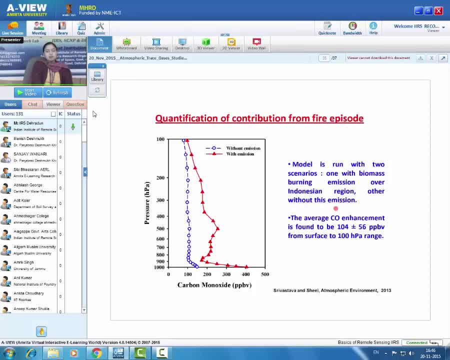 model, so model run with two scenario one model, so model run with two scenario: one with biomass burning emission over with biomass burning emission over with biomass burning emission over Indonesia region, other without this Indonesia region, other without this Indonesia region, other without this emission. so the difference is at each. 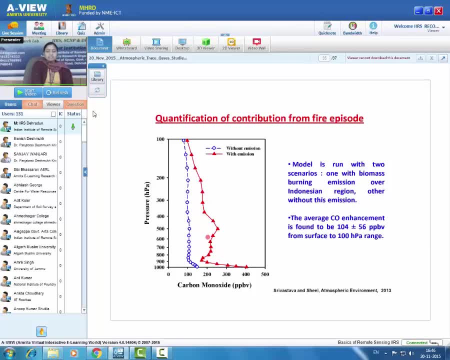 emission, so the difference is at each emission, so the difference is at each level can be calculated. we know that level can be calculated. we know that level can be calculated. we know that because of model we can calculate that at. because of model, we can calculate that at. 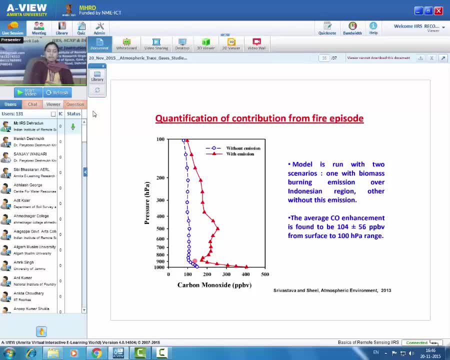 because of model, we can calculate that at each pressure level, how much amount of each pressure level, how much amount of each pressure level, how much amount of carbon monoxide is being added and the carbon monoxide is being added, and the carbon monoxide is being added, and the average is taken from surface: 200 hecta. 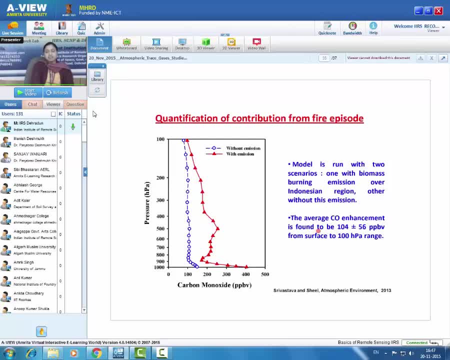 average is taken from surface 200 hecta. average is taken from surface 200 hecta Pascal, and we have found that average you, Pascal, and we have found that average you Pascal, and we have found that average you enhancement is around 104 plus minus 56. 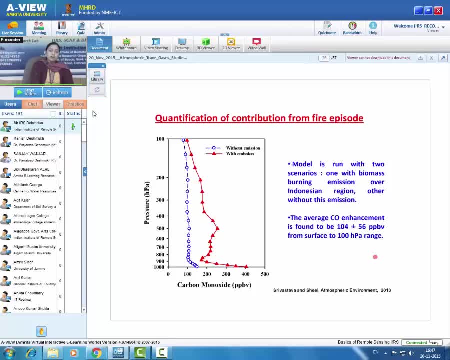 enhancement is around 104 plus minus 56. enhancement is around 104 plus minus 56 ppb. so we can quantify the contribution ppb. so we can quantify the contribution ppb. so we can quantify the contribution. we can identify the source we can quantify. we can identify the source we can quantify. 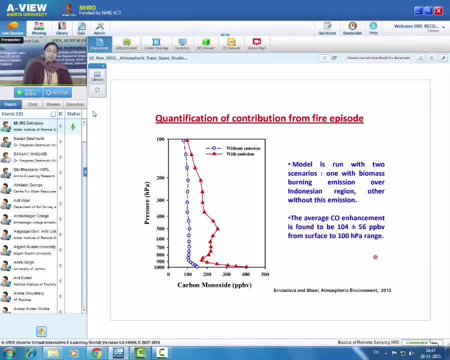 we can identify the source, we can quantify the contribution, when we utilize the contribution, when we utilize the contribution, when we utilize model, but model alone cannot work. we need model, but model alone cannot work. we need model, but model alone cannot work. we need satellite observations, also for the. 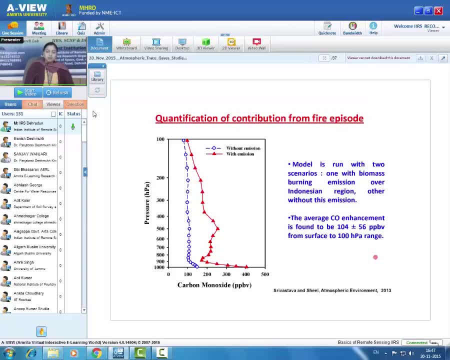 satellite observations, also for the satellite observations, also for the validation of model. so it can give you validation of model, so it can give you validation of model, so it can give you very important information when you very important information, when you very important information when you analyze satellite data along with 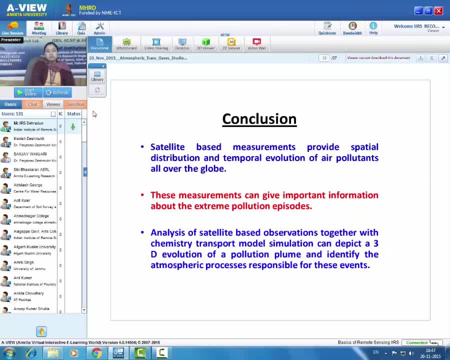 analyze satellite data along with analyze satellite data along with chemistry transport model. so conclusion: chemistry transport model. so conclusion: chemistry transport model. so conclusion: satellite based measurements. provide satellite based measurements. provide satellite based measurements. provide spatial distribution and temporal spatial distribution and temporal spatial distribution and temporal evolution of air pollutants all over the 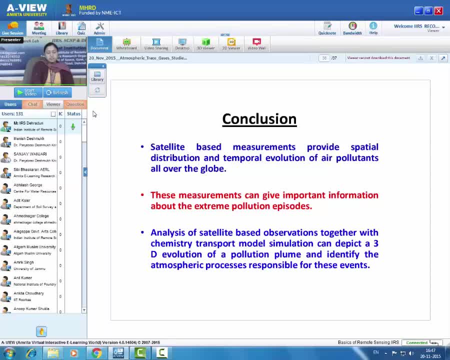 evolution of air pollutants all over. the evolution of air pollutants all over the globe. these measurements can give globe. these measurements can give globe. these measurements can give important information about the extreme. important information about the extreme. important information about the extreme pollution episodes. analysis of pollution episodes. analysis of 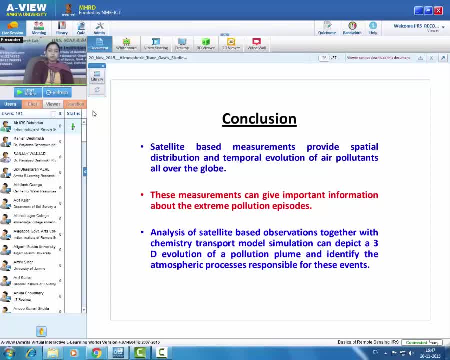 pollution episodes. analysis of satellite based observations. together with satellite based observations. together with satellite based observations, together with chemistry- transport model simulation. chemistry- transport model simulation. chemistry- transport model simulation can depict a 3d evolution of a pollution. can depict a 3d evolution of a pollution.